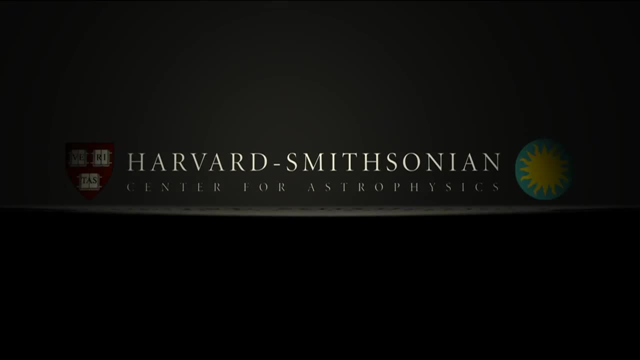 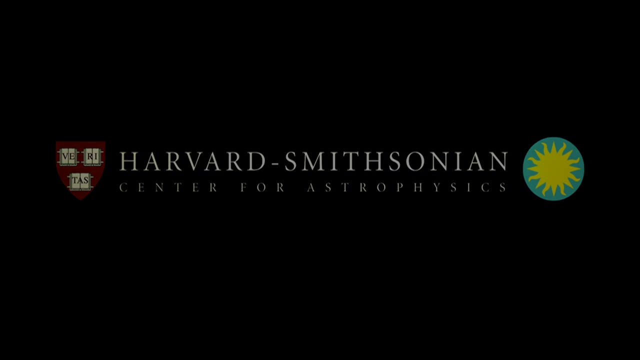 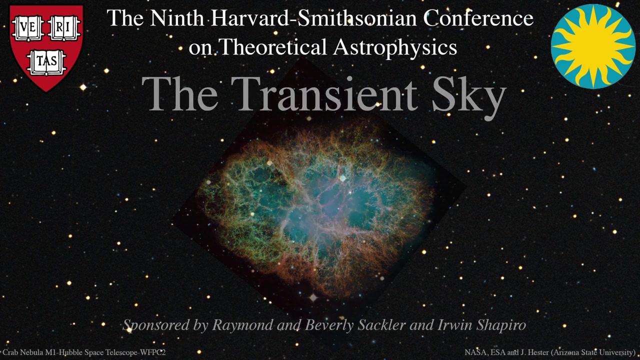 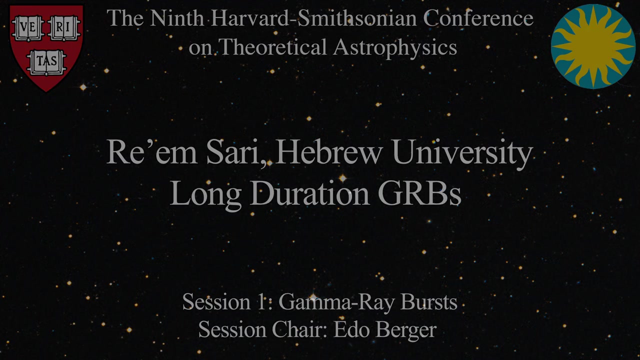 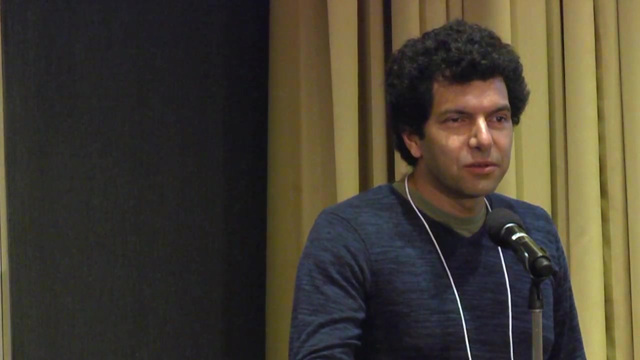 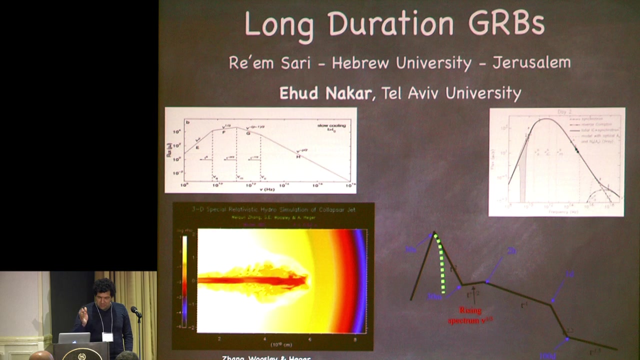 So good morning everybody. This talk was supposed to be given by Woody, but he's not feeling so well, so I was asked to substitute. Had he been here, I'm sure he would have given a better talk, but you have to suffer me. Okay, I was thinking I was asked to give a review about long-duration. 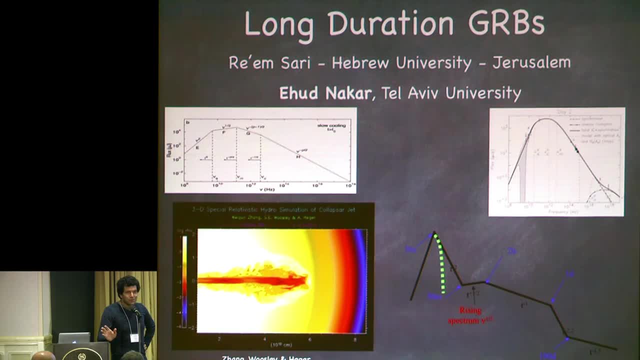 GLBs, and this is the first time I hear that this is going to be mostly observational, because it's not going to be. I wasn't told anything about that, So I'll go through a quick review of everything we know, or roughly the important thing we 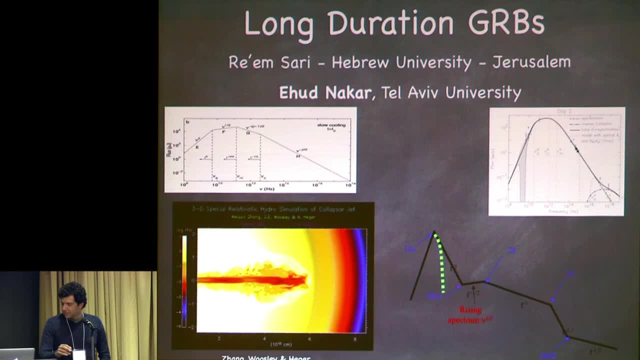 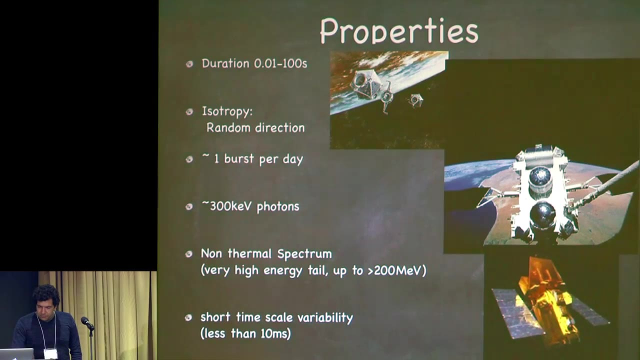 know about gamma ray bursts, long-duration gamma ray bursts, and then I will try to leave some time to focus on the things which are more controversial, that we know less of, that we're less sure of meaning there's more work to do, Okay, So I guess everybody knows. 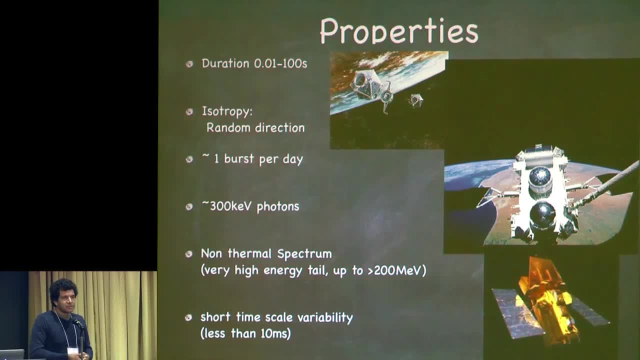 these properties. To give you a little bit of background of data, we're very excited to be here. We are very excited to see what European research affects our efforts, because we're very curious about how data can be used at the global level to demonstrate the power of gamma rays. 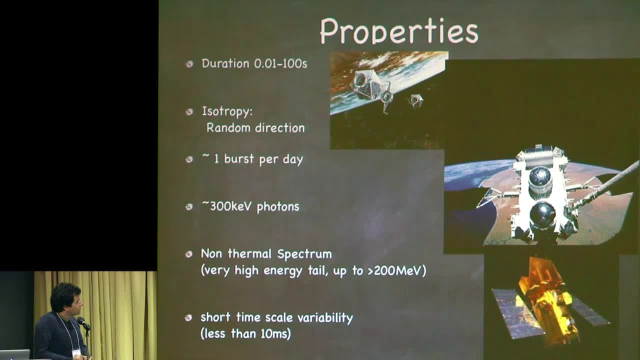 And we want to start with the safety of data. So these are the data that we're getting from NASA. Thank you, And I'll give you the links. So we cannot do research for the public at the moment, but we can do research at: 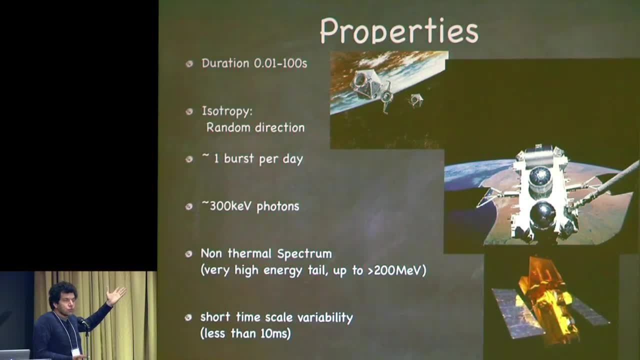 the global level, And so we can do research at the global level. They are short duration bursts. even the long ones are short. they last a few seconds, 100 seconds. They over the observable universe. there are a few of them per day. their spectra is: 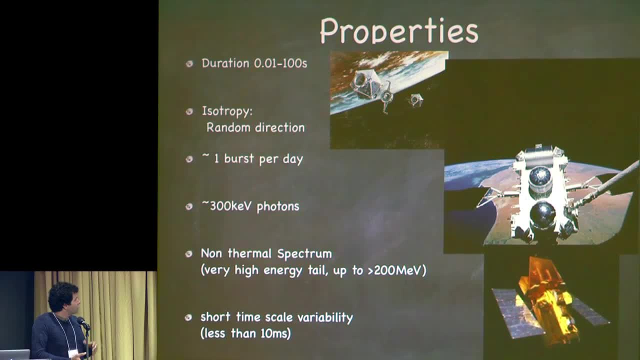 picked at around an MEV, slightly below, with some spread, but not too large. they're very non-thermal, both in the low energy tail and in the high energy tail. They have high energy tail going to GVs or more and they have very short time scale variability. 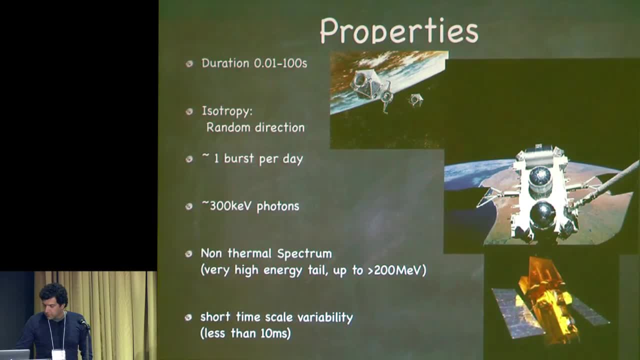 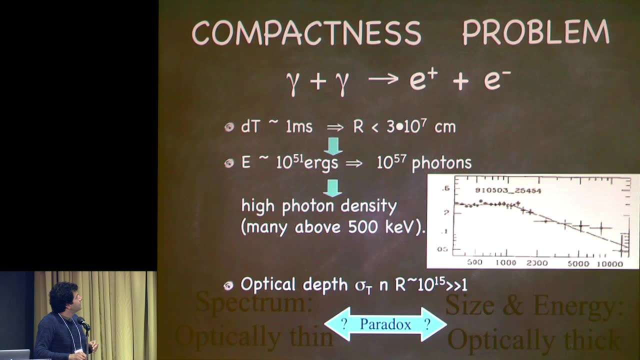 sometimes going down to milliseconds, more typically some fraction of a second. So this short list of properties immediately led to the understanding that there is a problem. Once you know that the distance to this object is cosmological, it gives you an energy of about 10 to the 51 ergs. 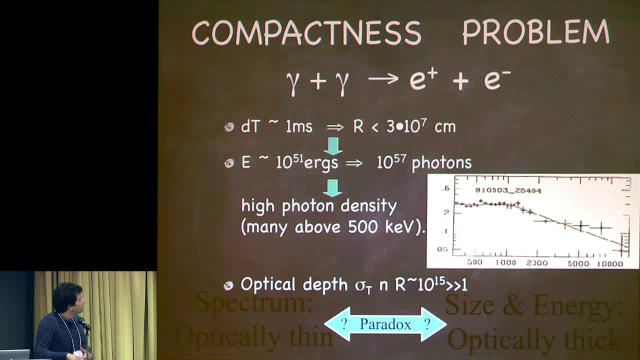 We know from different bursts it's somewhat different. it could go to 10 to the 54 ergs or 10 to the 53. With an MEV photon that gives you around 10 to the 57 photons. If you naively take the variability time a few milliseconds and you convert that by multiplying, 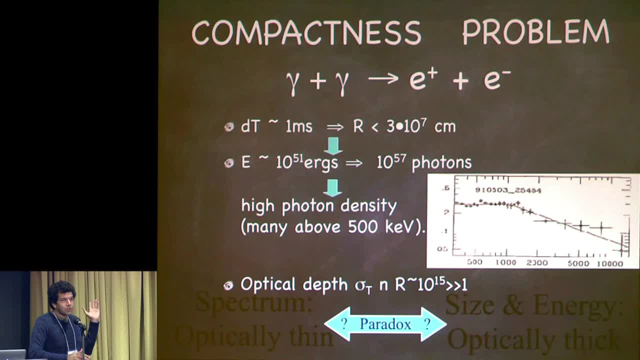 by the speed of light to a size, you get a photon density and you can calculate the optical depth for photons to leak out of this and the reaction that they can go is a pair creation to photons can create electron-positron pairs. These electron-positron pairs that just form can then scatter the rest of the photons and 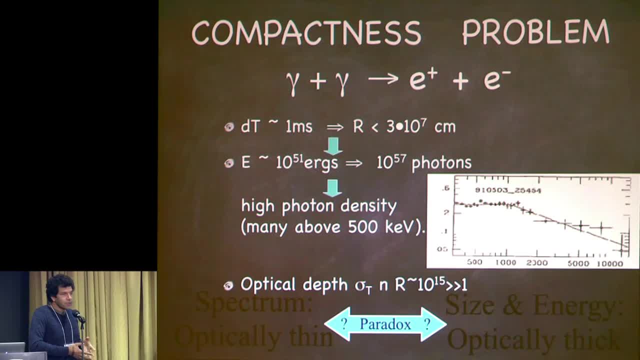 then they can go into the atmosphere. So that's what we're looking for. So we're going to look at the thermal density of photons and you'll get a very thermal spectrum in contradiction to the observations. So just this calculation shows you a paradox between the observed spectrum, which is completely 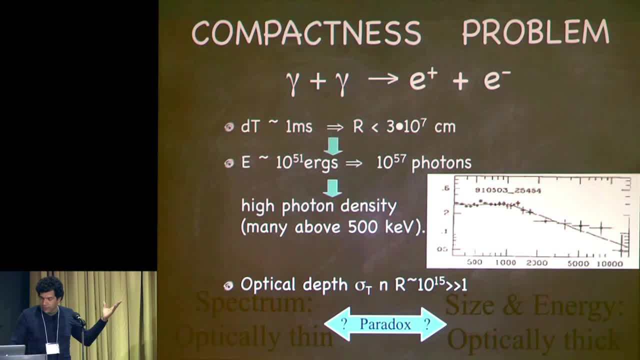 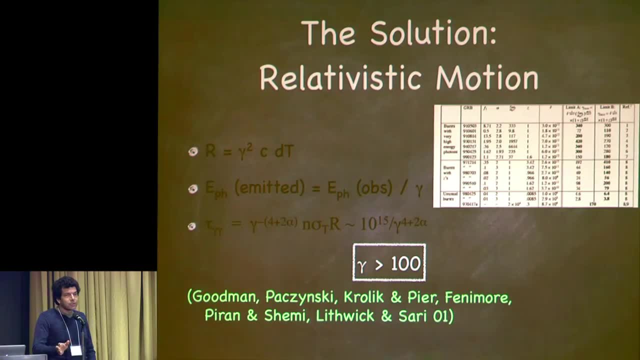 non-thermal and the theory that says that if this is the density of photons, it has to be very optically thick and therefore thermal, And there's basically only one solution that we all agree about. This is the thing that everybody agrees about gamma-ray bursts: is that relativistic motion? 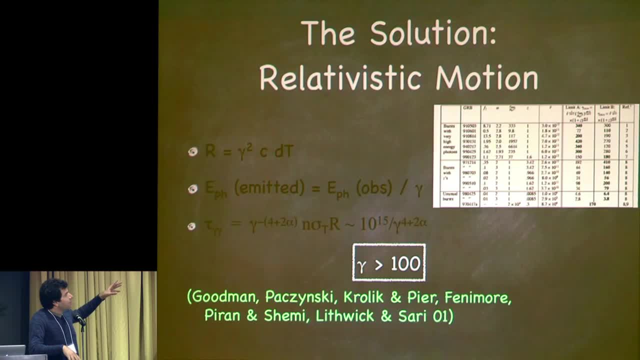 solves this paradox. When you assume relativistic motion- I'll come to that in a second- you can get a radius which is larger than the naive estimate of C times delta T by a factor of gamma squared. And since the radius comes square into the optical depth, you have four powers of gamma. reducing that optical depth. In addition, the photons in the source are much softer than the photons that you observe, So if you thought you were observing MEV photons at the source, they are much softer So they can't easily produce pairs. You need to go very high in the energy. So you can't easily produce pairs. You need to go very high in the energy tail. in the high energy tail to get the photons that can create pairs And that will reduce effectively the optical depth. So it turns out with a Lorentz factor of 100 or several hundred depending on the burst. 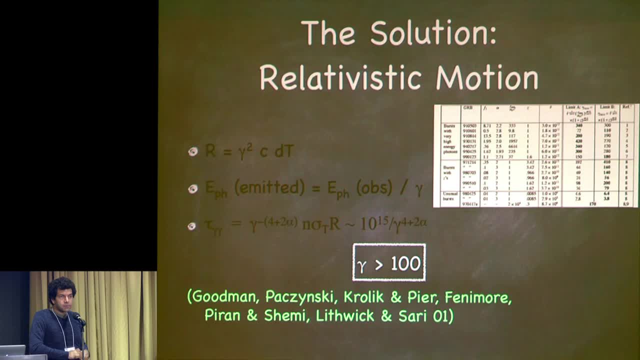 you're talking about. you can overcome this compactness problem And GRBs must be relativistic with about this Lorentz factor. There was some discussion what short GRBs are, if they should have the same kind of Lorentz factor or not. 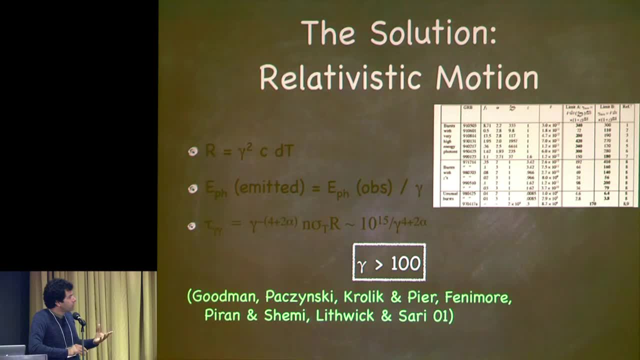 It turns out, they should have somewhat similar Lorentz factor. Maybe a little bit lower is also OK, And I think the record holder, for which we have very high energy photons, suggest that the Lorentz factor on at least some bursts is around 1,000.. 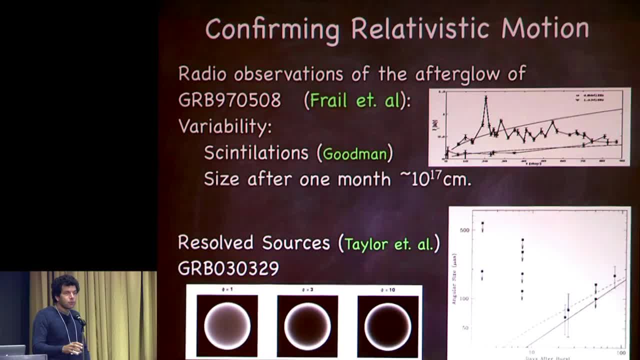 OK, Beside the compactness problem, there are many other confirmations of this relativistic motion. Already with the first afterglow We could say that the motion is relativistic. We could say that the motion is relativistic. We could say that the motion is relativistic. 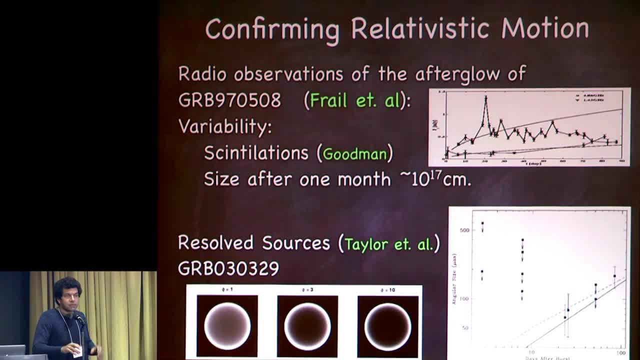 By several arguments, but maybe the most direct one is seeing the scintillation disappearing. So radio objects: they scintillate, and as the fireball expands it becomes too large on the sky And therefore it doesn't scintillate. 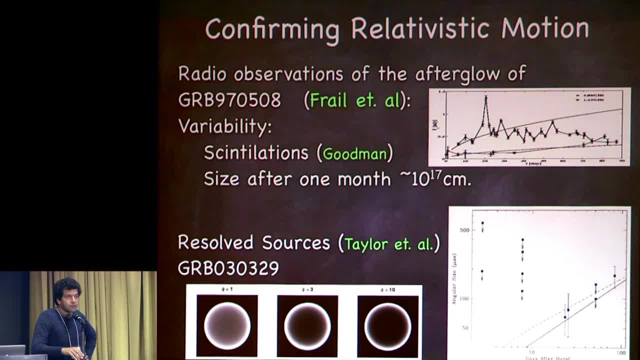 The fluctuations decay And that suggested the size of 10 to the 17 centimeters after about a month, which means relativistic motion. In some cases you can also resolve the source. This is the figure on the right. You can actually see the size of the source and it agrees again with about the same numbers. 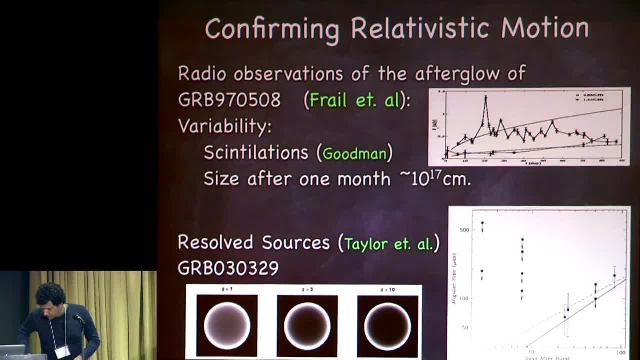 When we're talking about resolved sources from the theoretical point of view, sometimes in the future, I hope we can see some images like that. So this is what the image of spherical GRB should look like, if you could really resolve it. And actually, when we're doing scintillation calculations of gamma ray bursts, we have 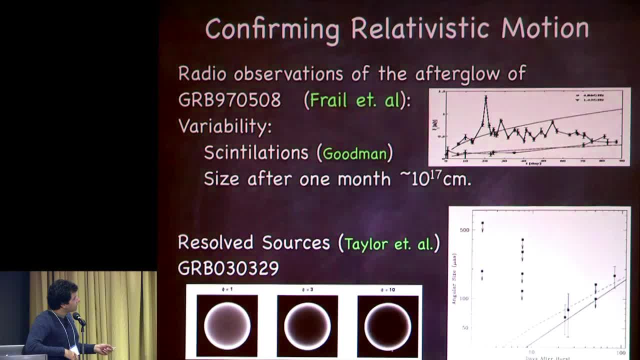 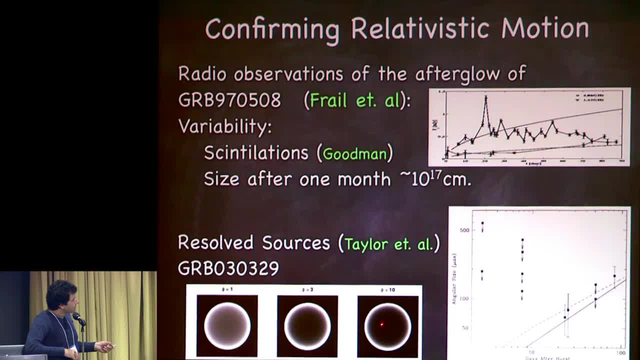 We have to take this. We have to take this- So this is the shape- into account. So you see that the high frequencies in the radio above the self-absorption frequency. You have a very narrow ring which is pretty dark in the middle. 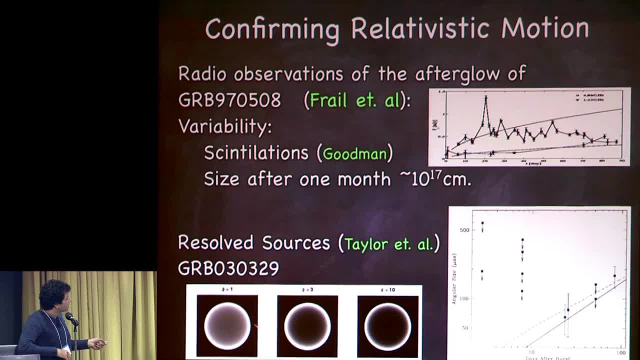 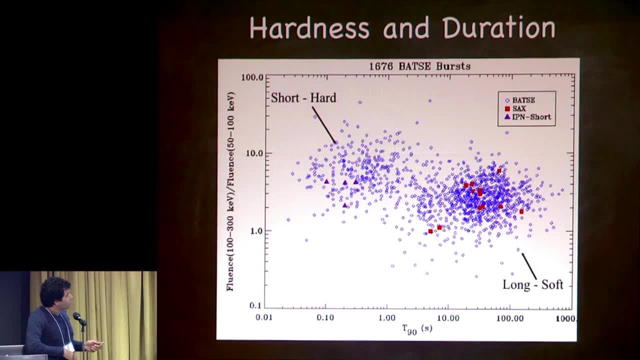 So this is what the theoretical images of GRBs should look like. At low frequencies, below the self-absorption, it's more uniform. OK, So I was asked to talk about long GRBs. There are short and long ones. This is a plot of some of the GRBs' duration hardness. 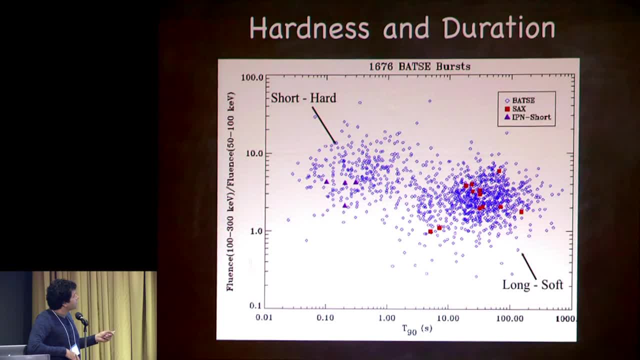 Hardness is the ratio between the mass and the time. And it's the ratio between the mass and the time, Hardness is the ratio between photons at some high energy band of Bazzi to the low one, And you can see that you can sort of see here two groups. 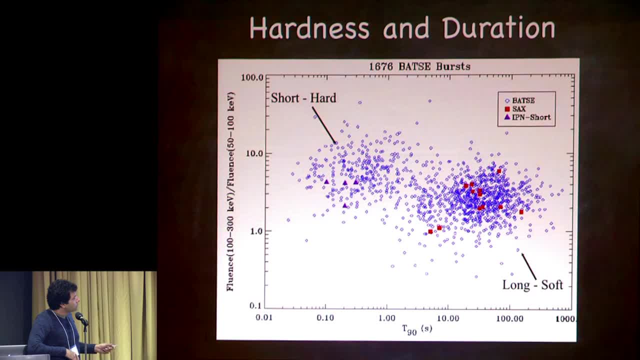 Long ones, roughly 10,, 20, 30 seconds, but spread between one and a few hundred, And short ones which are somewhat harder, higher in this axis and around 0.1 second. There is probably some diagonal line that you can put in here to divide between them. 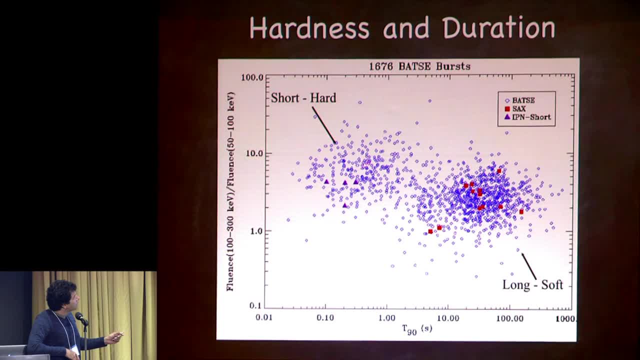 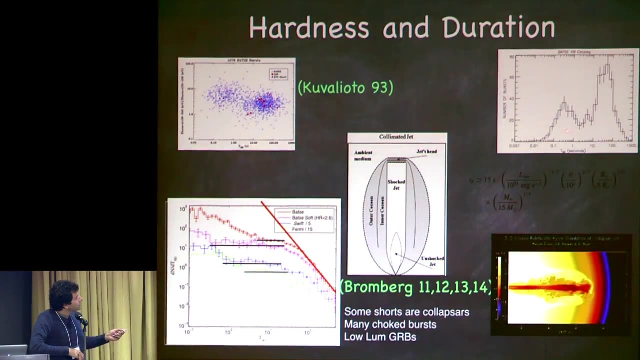 So as you go to bursts which you know are hard, they can be even longer somewhat and still belong to the short distribution. This is the original plot in which the short and the long groups were discovered. If you project that to the T90 axis- the duration of the burst- you can see that there are actually 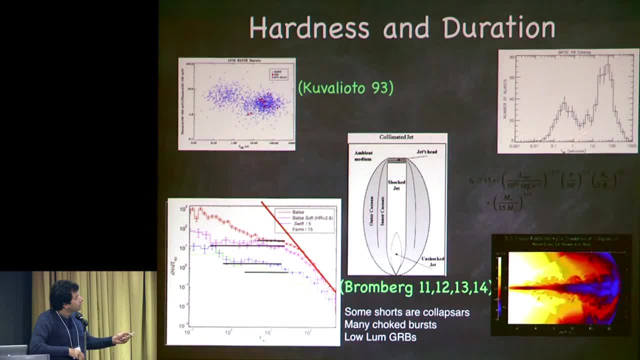 two humps And the dividing line between them around one second is the standard definition of short and long. This is kind out of KLB for glbs. In a series of papers with Bloomberg we calculated the interaction of a jet with a surrounding. 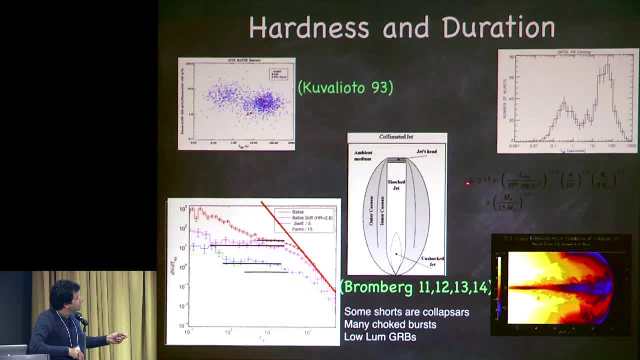 as we can see in this nice simulation, And we calculated that it takes about 15 seconds for the jet to come out of a star. It depends on the luminosity of the jet, on its opening angle, on how big the star is. Obviously bigger stars take longer, not completely linear with the radius, because the bigger 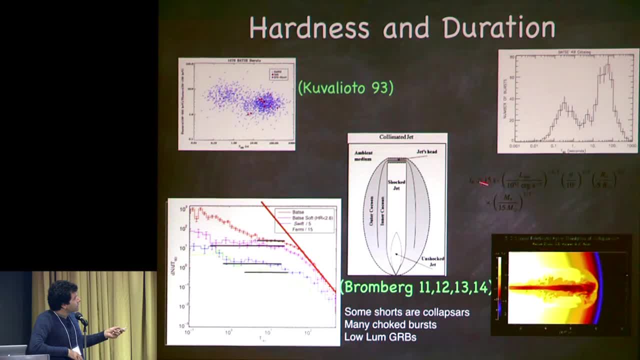 is, and it's easier for the jet to pass through, but it takes about 15 seconds. so we're trying to figure out how to get this distribution of duration, given that it takes 15 seconds for a jet to just come out of the star, so it must mean that the jet itself has to be active for more than 15 seconds. 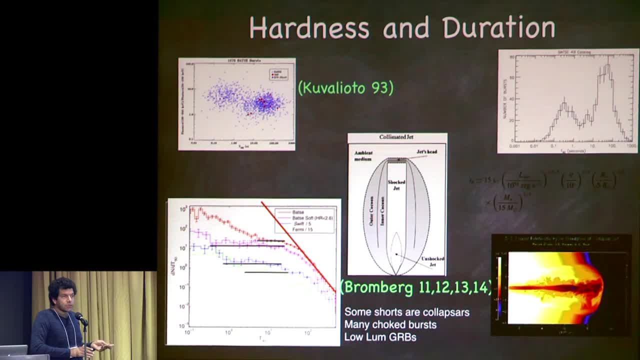 otherwise it will never come out and it means that we lose all the bursts that are shorter than 15 seconds. so the way to get bursts which are as as short as a second or two is to have a burst that, instead of a jet that works instead of 15 seconds, works 16 or 17 seconds, so that once you subtract, 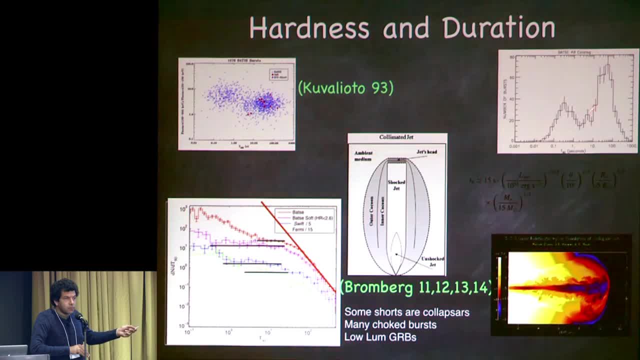 15 seconds, you have the one, two, three seconds burst that you're observing here. so the prediction that comes from that: if you have a distribution of duration, whatever distribution of duration, and you cut all the bursts which are shorter than something and you subtract that same number, the 15, 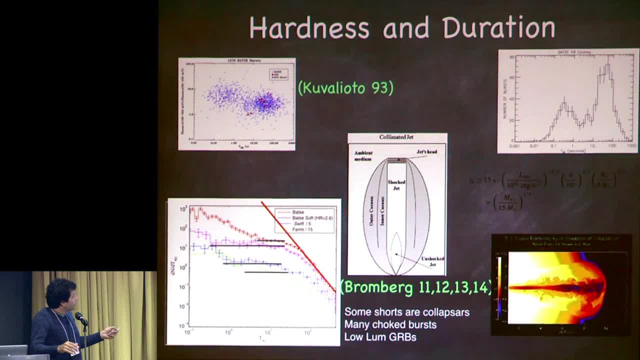 seconds from the length of all the others that you keep. the immediate prediction is that you get a flat distribution in dn dt, not dn d log t but dn dt of the duration distribution. so as soon as we understood that, we went to check and we seem to be compatible with that understanding. so this is a confirmation. 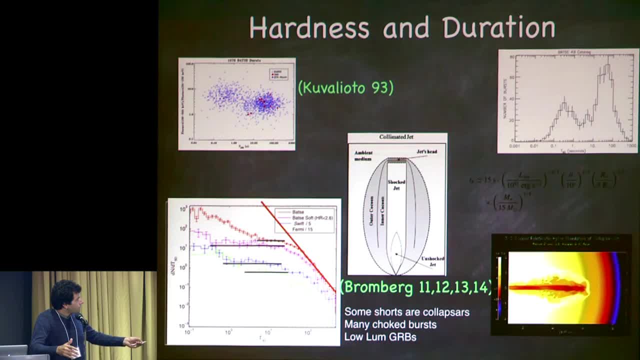 i wouldn't say it's a confirmation of the collapsor model of this jet picture, but it is a confirmation that there is, or a suggestion that there is, a certain time that limits the duration of the burst- and all bursts were probably longer, subtracting something from the duration of the 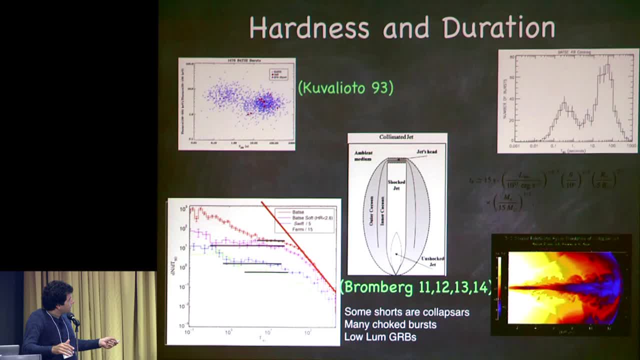 burst and all bursts were probably longer, subtracting something out of the real duration. now it also means, if you, if you look at the distribution of duration above this- uh, 15 seconds, you see a very strong parallel. so there are only a few bursts which are much longer than that, and that suggests 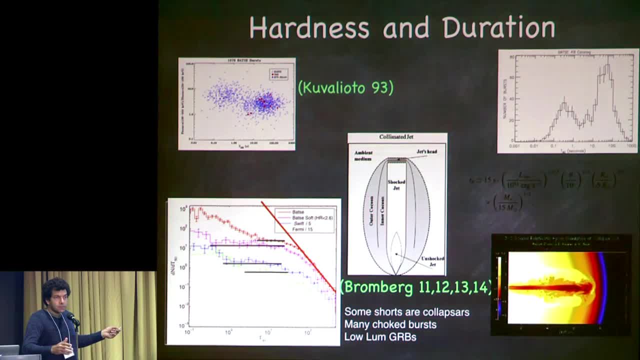 also that the number of bursts which used to be shorter than 50 seconds but disappeared is large. so maybe there are many, uh, choked bursts, if you take this extrapolation seriously, and maybe we'll make some connection with low luminosity jibbies in a few minutes. 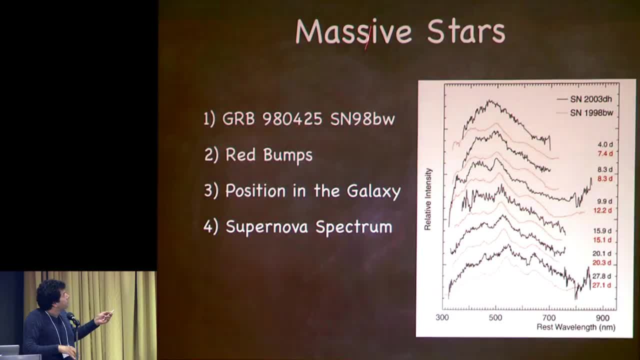 okay, we all know that there are, uh. most of the gamma rebirths come from massive stars. the long gamma rebirth comes from massive stars. there are many evidence for that, starting from this coincidence with some supernovae in 98, with theoretical understanding that collapsors may. 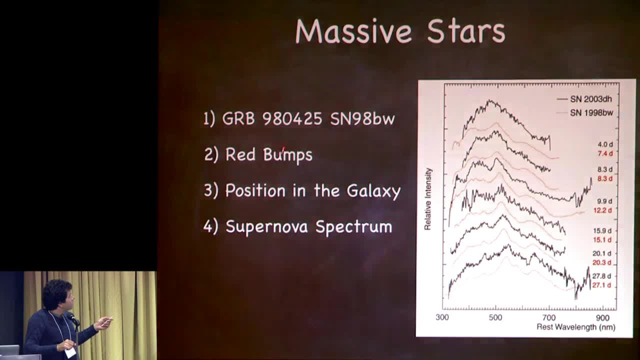 be able to produce gamma rebirth with red bumps in many more events which you can't really see. the whole supernova position in the galaxies and the type of galaxies, uh, the existence suggests that they are well associated with star formation, even more associated with the star formation than the star formation is, uh, and in some cases you can actually see the supernova. 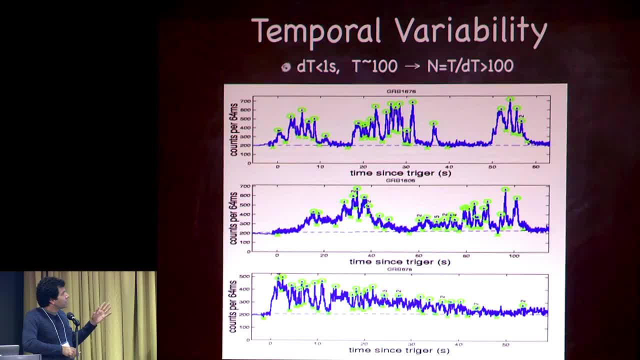 spectrum. one of the great clues that we have about the whole mechanism of gamma rebirth is the variability we see. we see short time scale variability of less than a second, as i said before, sometimes a millisecond or 10 millisecond, while the burst itself lasts 100 times longer than. 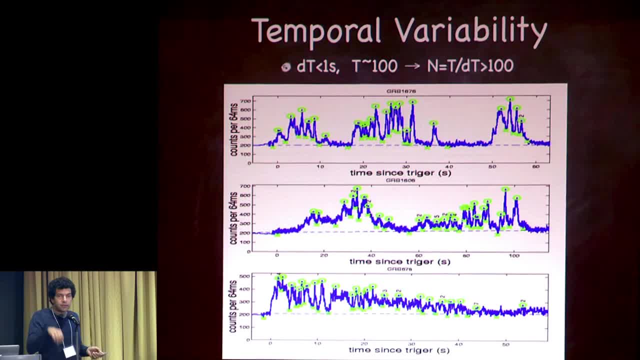 that and it's this large ratio between the duration of the burst and the variability that is uh interesting. so i took here some of the more variable bursts from the batzi catalog and i marked the peaks and you can see that the between the peaks the uh emission goes all the way to the background level, almost there, sometimes with big. 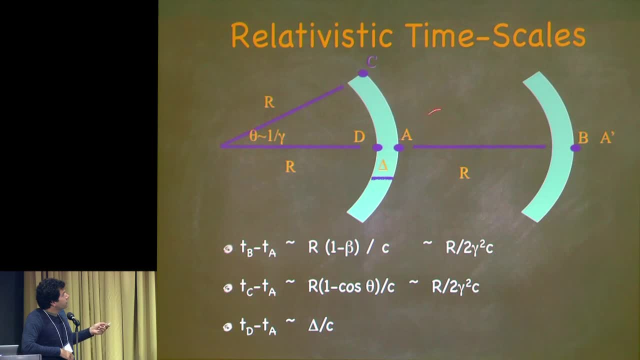 gaps when you think about the- uh relativistic time scales that are involved. there are two time scales which are equal in this problem. so if you think of something, let's say this shell that came out from an explosion that occurred in the origin here and at this point it, 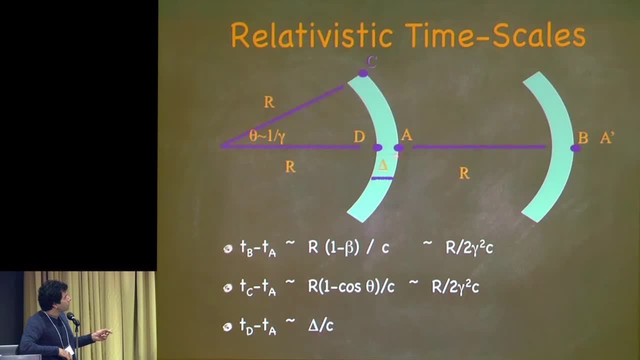 emitted some photon and then, some later time, it emitted another photon, while it doubled its distance from the origin. so it was initially at r and now it's at 2r, where it emitted photon b. there is some distance between photon b and where photon a managed to propagate to. this distance is 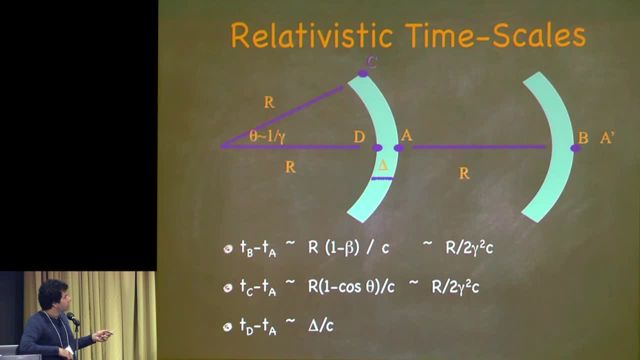 very short, because the shell itself moves almost at the speed of light, so they almost catch up with each other. but you can calculate what's the distance between them. it's the difference between the speed of the shell and the speed of light and therefore, uh, this distance between these two photons will give you some effective duration of. 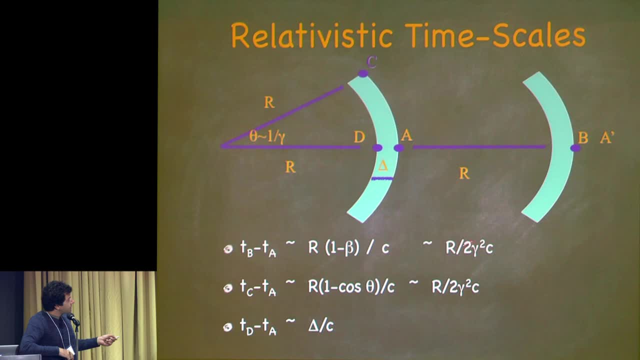 the burst which is about r over gamma square c, and the surprising thing is that this time scale appears in another, uh, geometrical thing in here, which is the difference in arrival time between the photon on the line of sight and the photon off the line of sight. now you can only go off the line. 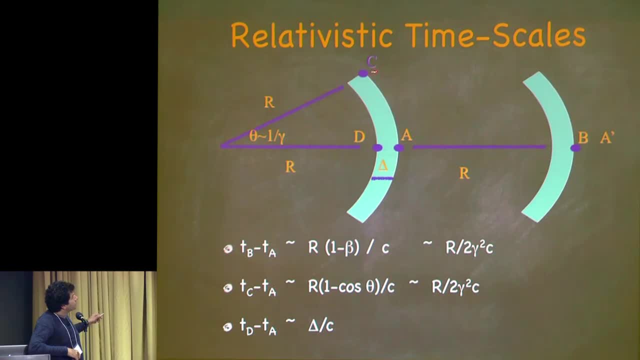 of sight about one over gamma in angle. because of relativistic beaming, the photons that are emitted from here are going mostly in this direction, plus minus one over gamma. so this guy just barely makes it to the observer but the photon that would have been emitted in here 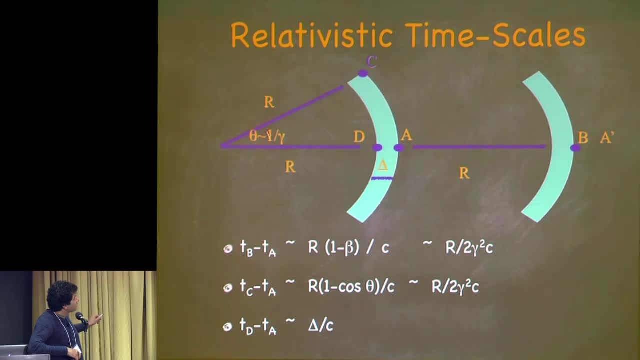 all the photons would go in there and you wouldn't see them. but within the opening angle of one over gamma, you can also calculate the delay time between photon emitted at a and at c, and it comes to be about the same thing. so what we call the angular spreading time and just the fly time are 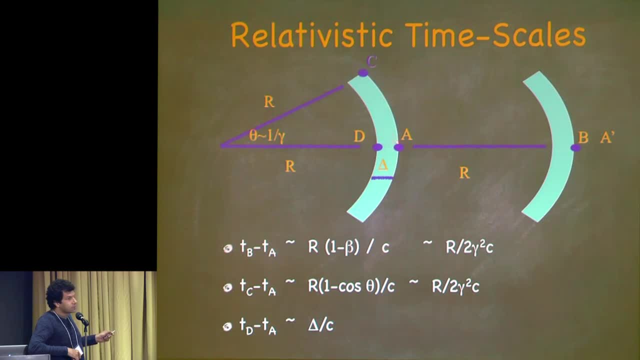 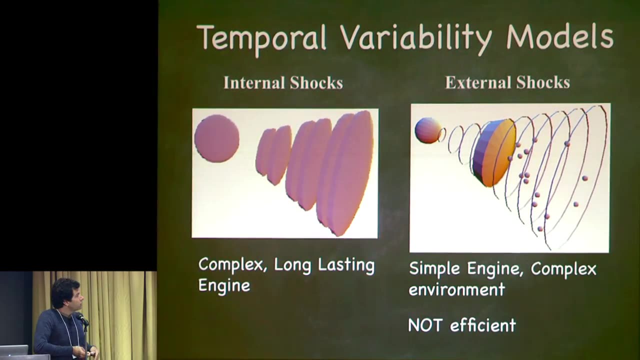 about the same. so that means that every signal that you have is being smeared on this time scale. so if you have a variable temporal profile that i showed you before, if you were trying to do that with a variable surrounding, so you make the surrounding from which the uh explosion is. 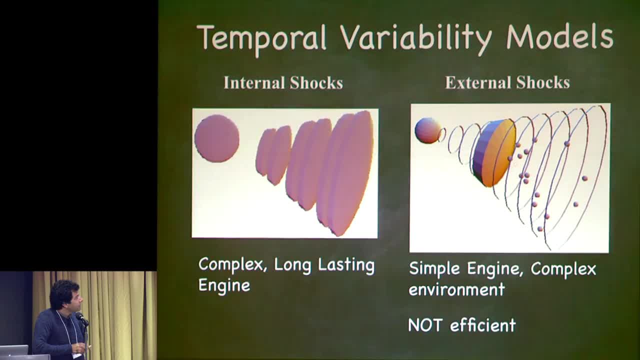 colliding with interacting with clumpy, it turns out that these clamps have to be extremely tiny to avoid this angular diameter problem, and when you do them so tiny, the fraction of the explosion that actually hits any of these clamps is tiny and the whole process becomes inefficient. 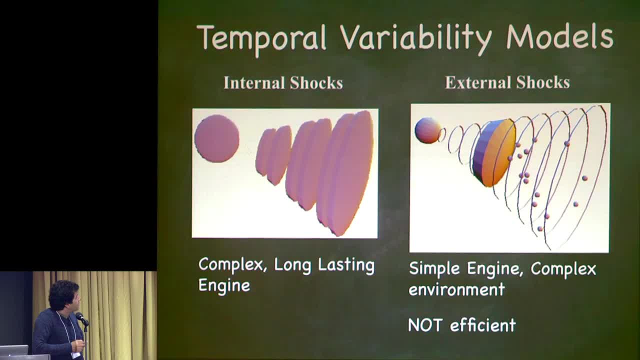 so the alternative that i think most people now think is the right thing is that the object itself is variable, so you can't blame the variability on the surrounding, because you have to make these clumps too small and it's inefficient. the object, the object itself, is variable, so that's. 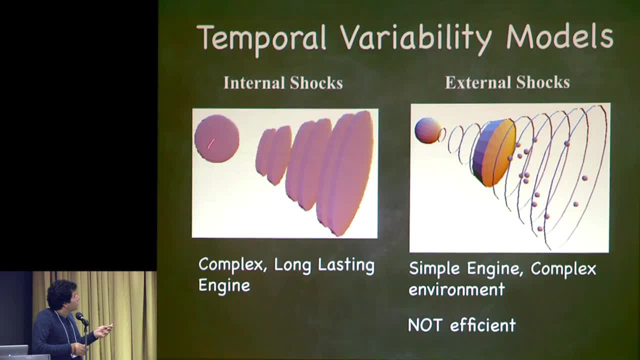 a huge clue on what is the source is doing. it has to be of a long lasting, maybe 100 seconds, with a variability of less than a second. and the story now, let's say, with the collapse of model, is that you form a black hole and then you feed the black hole erratically afterwards. 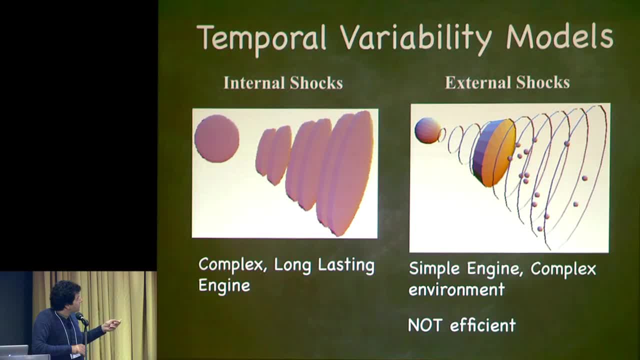 with uh, some accretion disk that is somewhat unstable, producing uh, all these uh shells which then collide internally between them rather than with the external environment. this some people claim that this process is also inefficient because after the shells collide they're still moving, so they still have some kinetic energy left after the collision. but if you look at in details it depends. 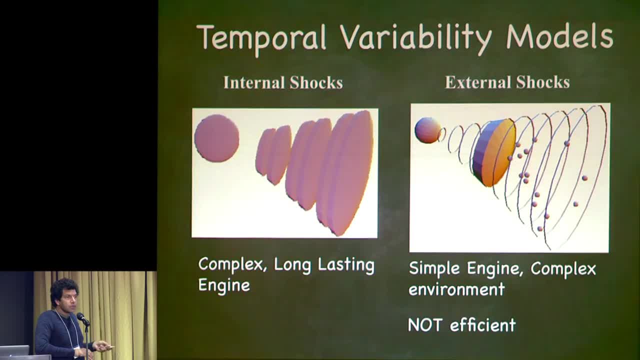 on the ratio of florence factors between shells. so if you assume that the shells have comparable lawrence factor, yeah, then the efficiency of this process is 10- 20 percent. if you assume that the ratio of florence factor is huge, you can get to 100. there is no actual uh limit in here. 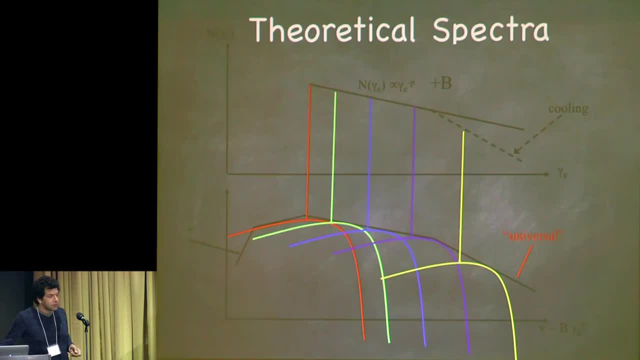 okay, let me skip that. i think i said that this is what we think, the stages that long grbs are forming from now about spectra. so we think, uh, that gamma ray burst form. both the gamma ray burst and the afterglow are produced by synchrotron radiation. 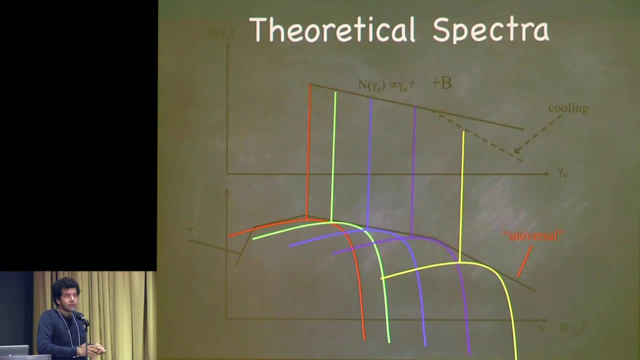 if you take a parallel distribution of electrons, presumably accelerated at the relativistic shock- let's say this to some- power minus p, roughly two, slightly more, and you put it in a magnetic field, you have all these electrons radiating. each electron has its own spectrum and when you sum, 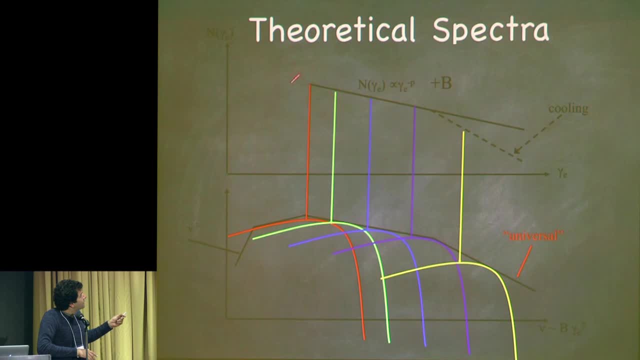 them all up, you get this uh broken power law, despite the fact that you started from one single power law, because there are some other mechanisms that produces break breaks. so one of them is the cooling break. when you go to high enough frequencies, the electrons cool. so, even though you injected them. in that rate the actual number of electrons that survive in any given time at high energies is smaller, because those guys cool. so that provides this break. there is a minimum injection energy, so below that we get the low energy tail of synchrotron radiation. we'll get to 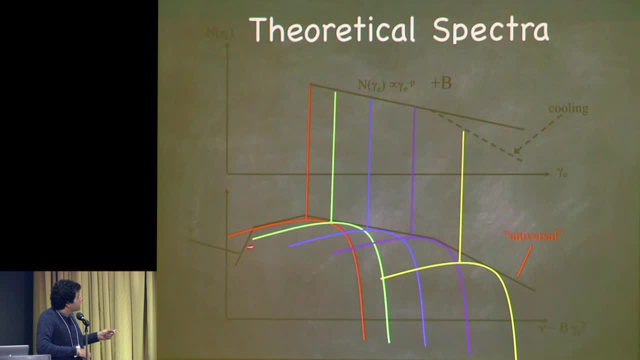 that in a second and at very low frequencies you have self absorption. so you have a new square, or new to the 2.5, depending on the circumstances- spectrum. So we get these four broken parallel segments out of a single parallel distribution of the electrons. Now, supposedly this should have been the 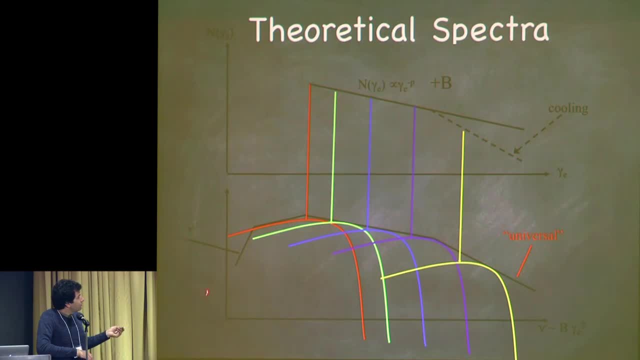 spectrum, both in the afterglow and in the gamma-ray burst itself. We all know this is the spectrum in the afterglow. We model most afterglows according to this kind of spectra. But if you look at the burst itself it doesn't seem to fit the 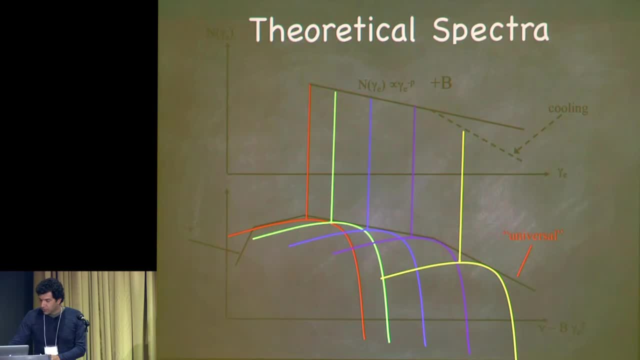 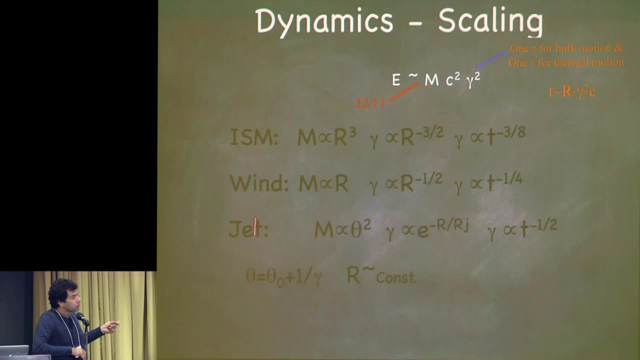 spectrum in the gamma-ray burst itself. So this is still a puzzle we have to work on. During the afterglow we can work on how the shocks evolve when they collect more and more material. Basically, conservation of energy, more or less the fraction of 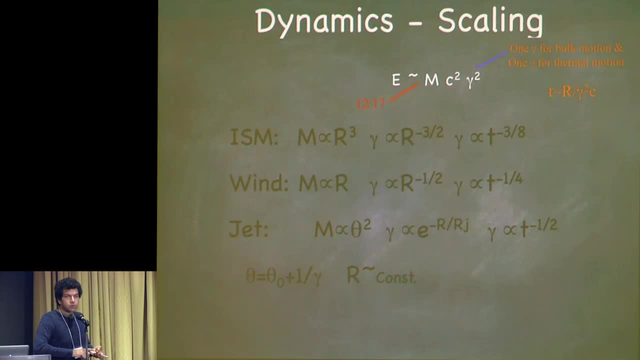 energy that is emitted is limited, both because of cooling that is not completely efficient and because the fraction of energy that is going to the electron is not unity and you can only radiate that. So if you assume that the energy is constant or you take some variation of this, the energy is about 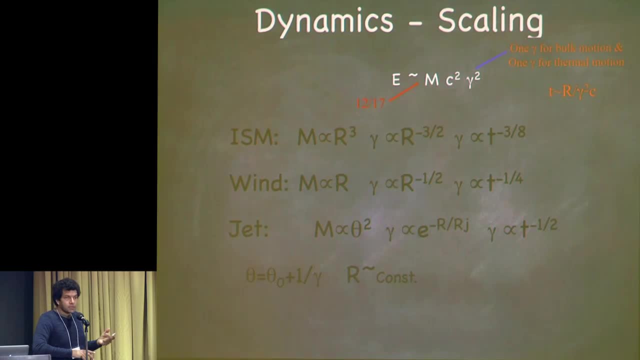 the mass times, C square times. the Lorentz factor: square. The reason the Lorentz factor here is square is because you have thermal Lorentz factor of the protons in the fluid and a bad Lorentz factor of the whole thing. So that's why you get a square. And now, if you put some thing for 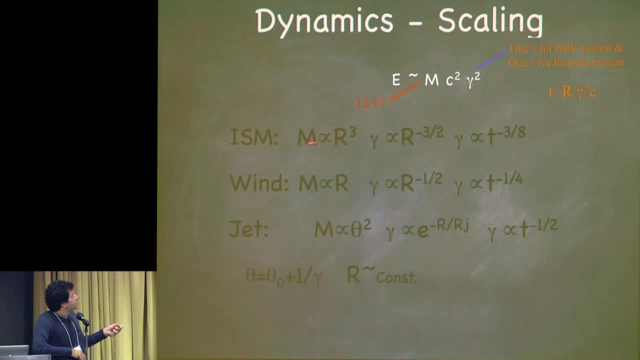 the mass. if the surrounding has constant density, the mass goes like the radius cube. If it's wind, it's only proportional to the mass, to the radius. And if you plug this in here and you take the relation we just discussed between time, radius and gamma square, you get all these relations. for how the 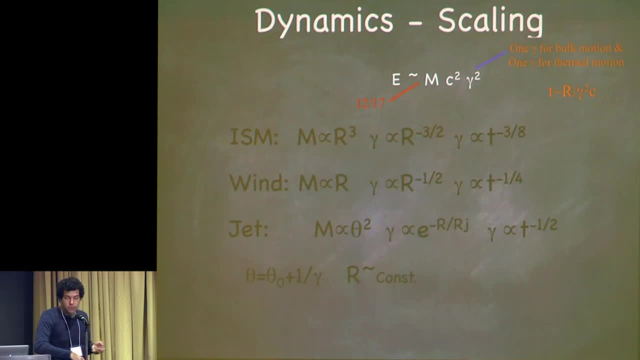 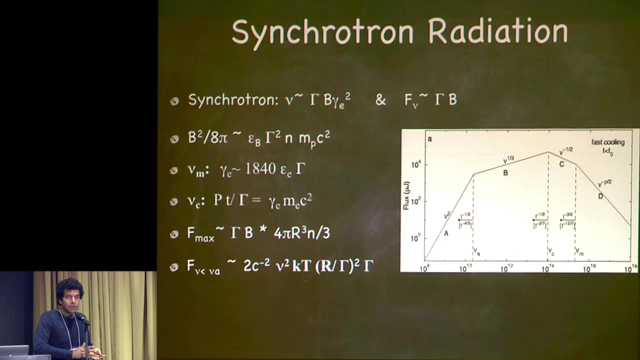 Lorentz factor evolve in time, how the radius evolve in time, and therefore you can calculate all these breaks In the spectrum and see how they evolve. and this gives a description of the afterglow that is roughly, I would say, in agreement with what we observe on long. 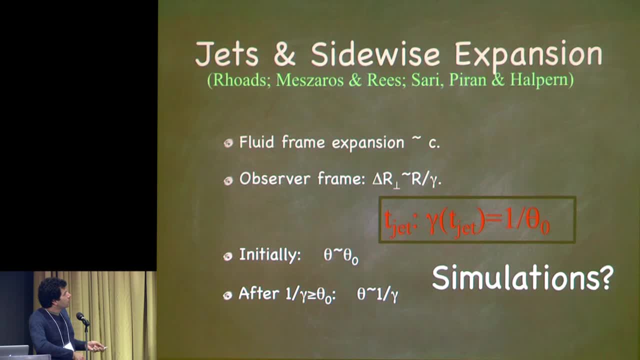 GLBs afterglows Jets. we believe that the emission coming from GLBs is collimated, Especially, it seems to be true for the highly energetic GLBs. This was suspected already, if not more than a year ago. But it seems to be true for the highly energetic GLBs This was suspected already, if not. 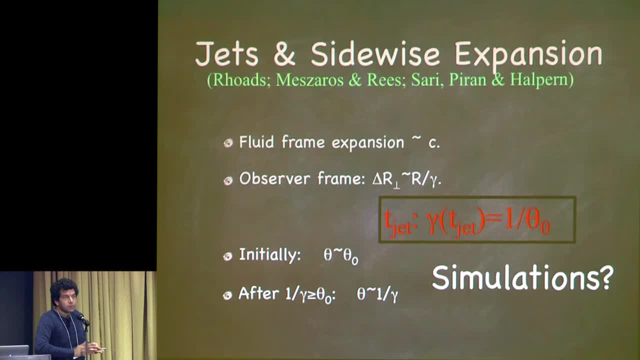 just from the energetic point of view, because the energy is so large, maybe it's collimated, And also from the fact that we understood that the explosions are relativistic, so we can't see the thing that is not directed to us, So we don't know if it's there or not, so we might as well assume that it's jets. The. 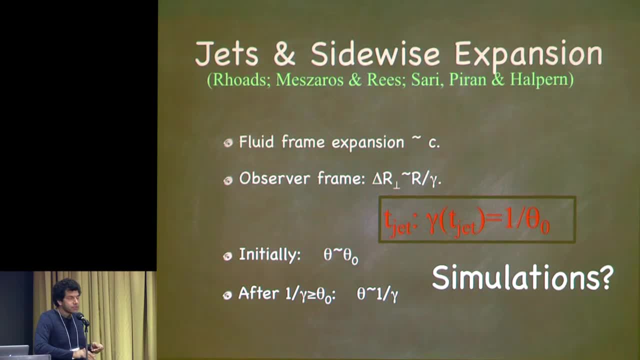 confirmation came from the fact that we saw the light curve starting decaying faster after a while. And this is because if the fluid expands in its its own frame roughly at the velocity of light because it's relativistically hot, then then when the low is factor of the whole, ejecta decelerates below one of the 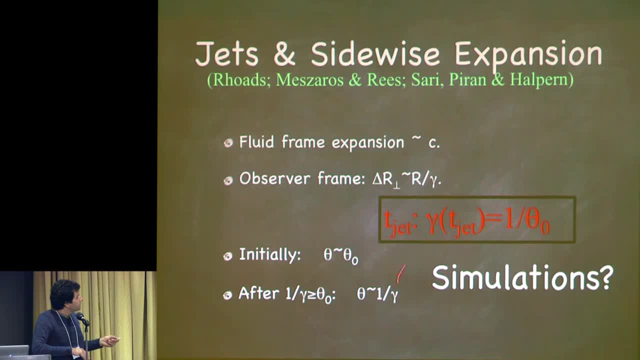 opening angle of the jet, you'll have sideways spreading in the faster decay of the light curves. Numerical simulations of these business have been zigzagging. You can tell us what the latest stuff is. So initially, Andrew used to come tell me: you know you have all these theories, but we run it in the 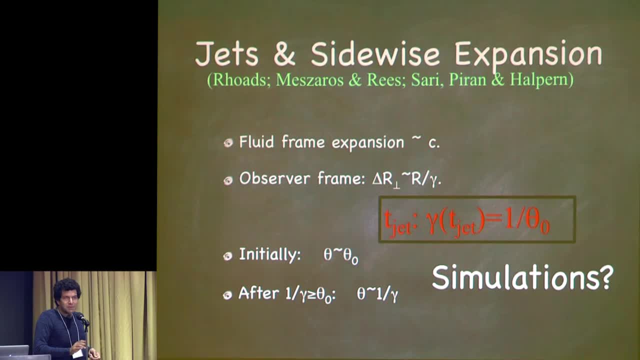 simulations the jet don't really spread. it doesn't work. Then I think some of the theorists also zigzagged. they said, yeah, maybe we can make it not spread. and then Ando said, oh, but maybe it does spread in the simulation. so 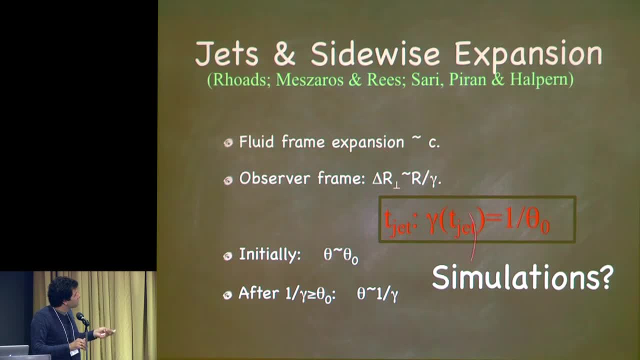 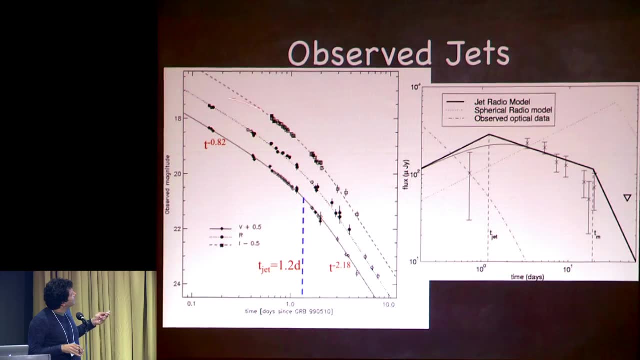 okay, I couldn't know how to make it not spread, so I think this is what it should be and everybody will catch up, hopefully, Okay. So yeah, this is the steepening I was talking about at some time. and for measuring this: 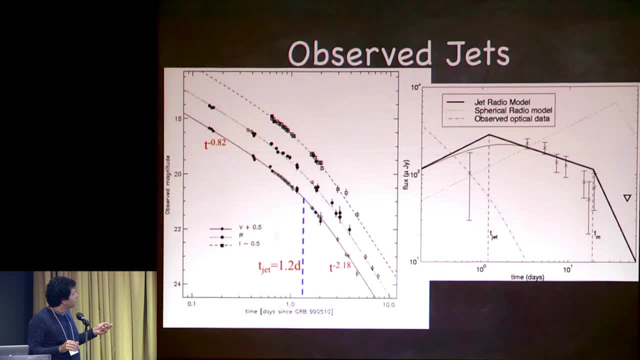 time you can tell what is the opening angle of the jet. A jet break at about a day tells you a Lorentz factor of slightly less than 10.. Later, slightly less than 10 at this time, meaning an opening angle of about. 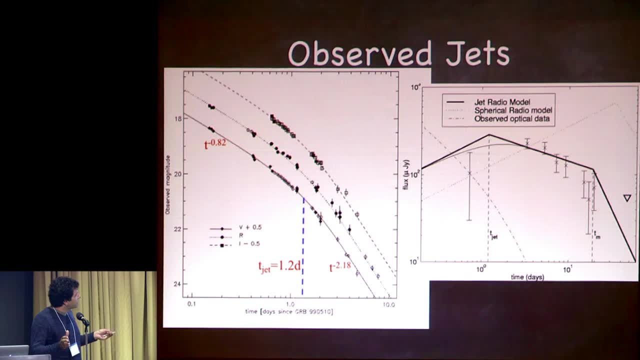 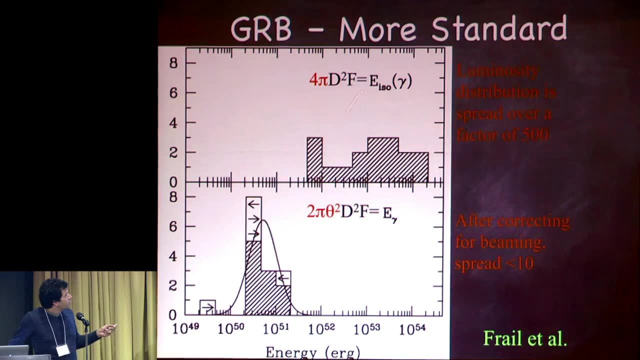 0.1 radians of the jet. So the timing of the jet gives you the opening angle and that reflects on the energetics and on the rate, basically, of these events. When you correct, this is a very old paper. 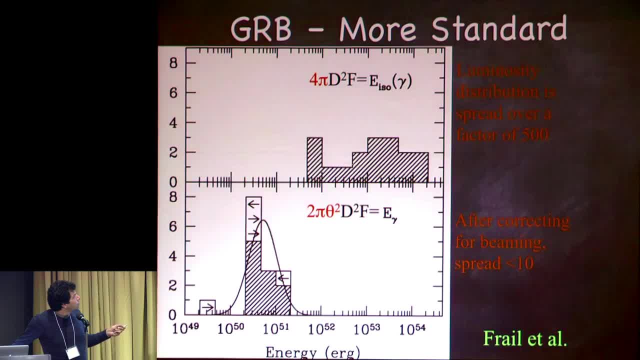 if you correct for the distribution of isotropic- seemingly isotropic- energies for the jet, they seem to have obviously smaller energies but also more concentrated energies. It doesn't seem as good as this, but still it seems to be okay. 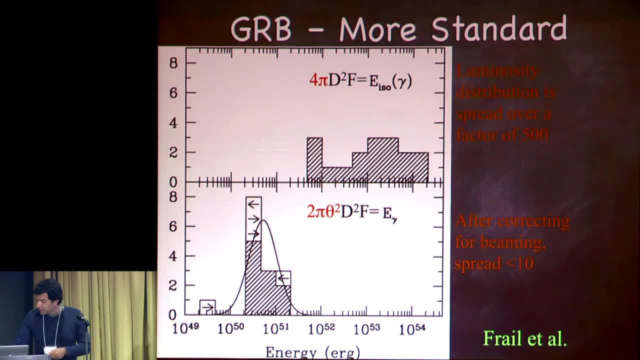 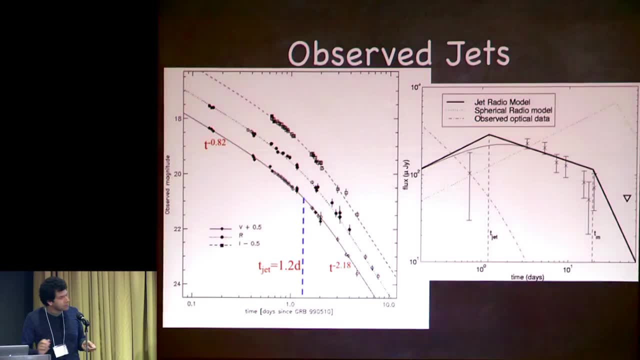 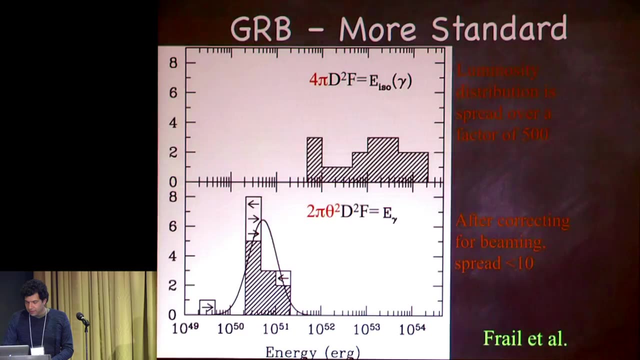 The latest time with this? well, the latest thing with this burst is that, with the SWIFT data, we have somewhat less clear view of these jet breaks. Not always we see them, So I think the picture became more murky in the last few years than it used to be. 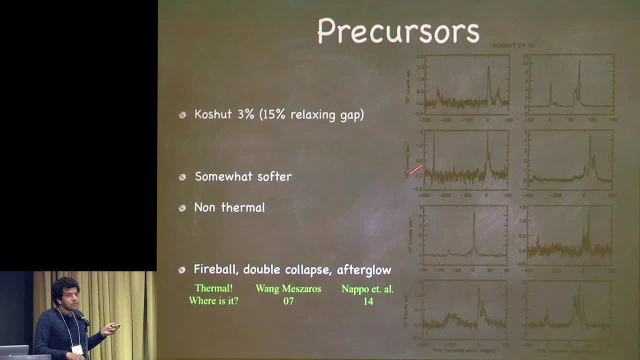 Shortly I will mention precursors. I think this is a big clue that, first of all, the precursors haven't been harvested yet. Precursors, they appear in 3%, if you define them one way, or 15% of burst. 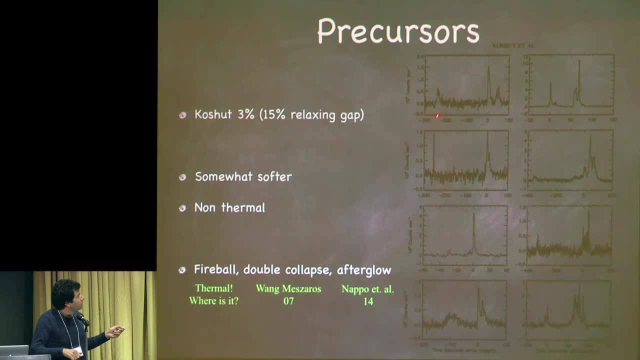 It's some emission that is weaker from the burst itself, well separated from it by background emission. It's somewhat softer, but still non-thermal, So we have to understand what it is. There are several models. One of them is that these are the emission from the 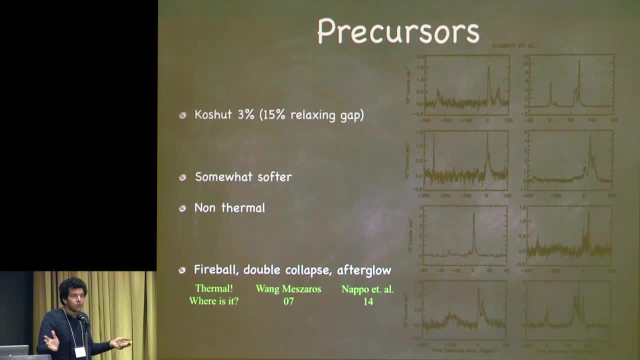 fireball itself. as the fireball expands and the original photons of the fireball leak out, you will get a precursor. So I think this is true. There should be this event, but these precursors are not completely thermal, so that 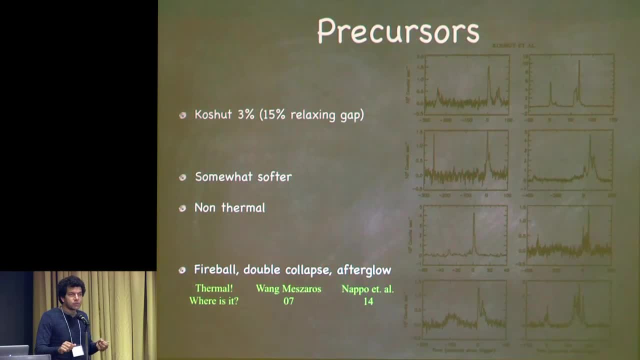 doesn't work. On the other hand, where is that thermal precursor that we do expect that should come out of this? So I think we have one precursor that we know should be there, that we don't see, and another precursor that we see. but 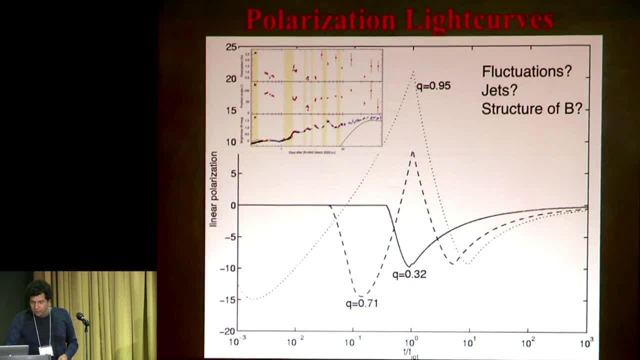 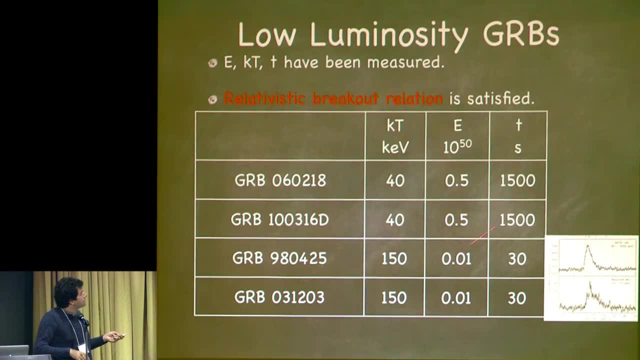 we don't understand. Okay, Polarization, let me skip that. if I'm so much out of time, Let's go back to talk about low luminosity GLBs. This is an exciting thing because it's a new class of objects. 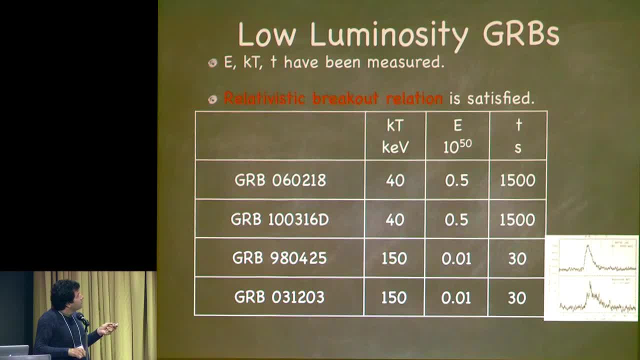 and I think they're quite different than the gamma-ray bursts themselves. They don't form by this direct jet that we talked about before. So this is a class of GLBs. Some of them are quite long, Some of them are moderately long. 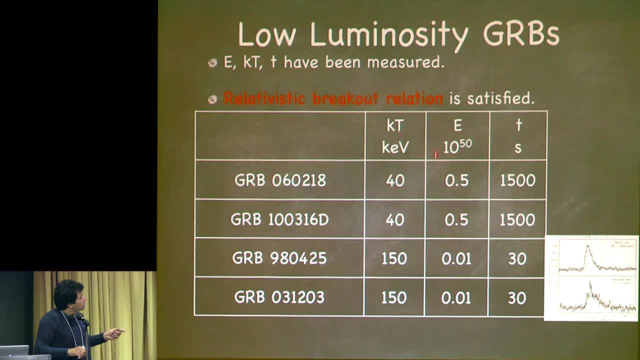 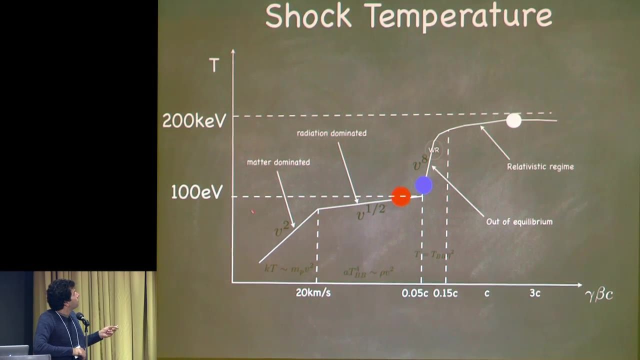 They have relatively low energies- This is what defines them- less than 10 to the 50 hertz, And this is a spectrum which is somewhat soft. So we think these are some kind of breakouts from a relativistic shock. So this is more. 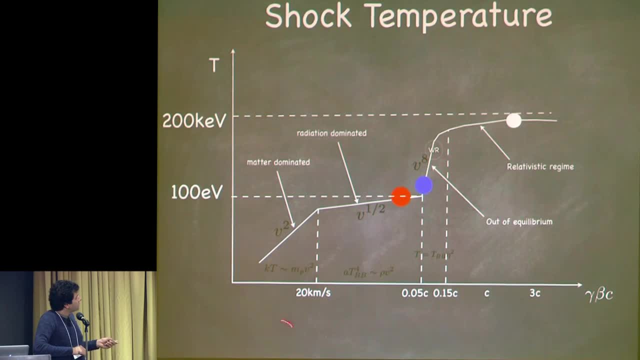 thermal emission than what we know in gamma-ray bursts. This is a figure of temperature that you expect from photons coming out of a shock as a function of the velocity of that shock. So initially you have some equal partition between the radiation density and the matter. 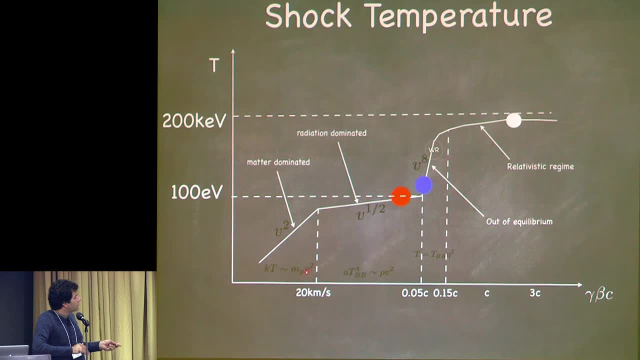 It goes like the velocity squared for low velocities, when the radiation is matter-dominated. So kt is important, v squared Quite. at small velocities you get radiation becoming important and then 80 to the 4 is equal to v squared and you get a very flat. 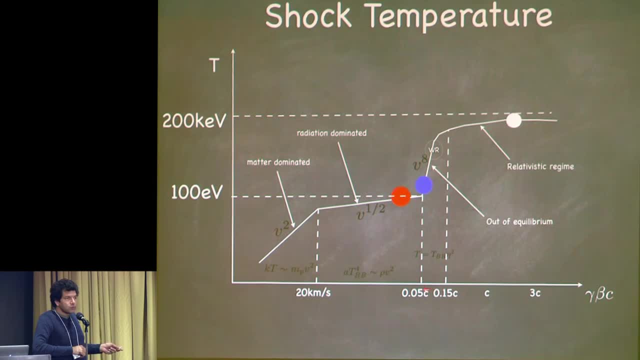 dependence. But then when you get to some fair fraction of the speed of light, the creation of photons behind the shock is not fast enough to create all the photons that are needed In order to arrive to thermal equilibrium. So had you been in thermal equilibrium, 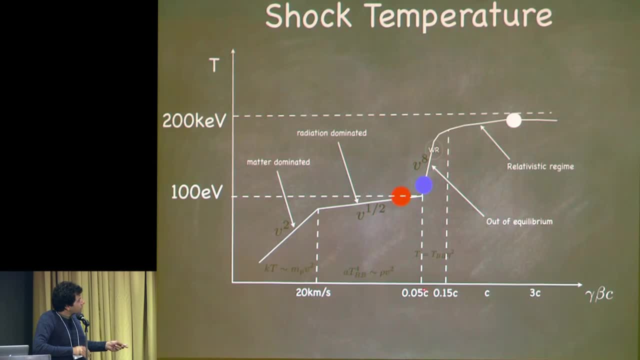 you would get these small temperatures, But for velocities which are higher than that you get way out of equilibrium And we think some of the explosions relevant to both gamma-ray bursts and definitely those low luminosity GLBs are of this type And therefore 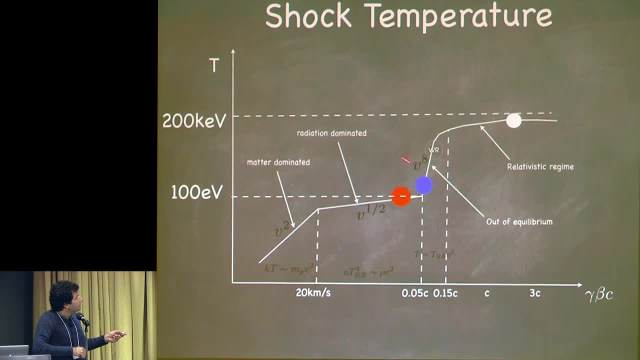 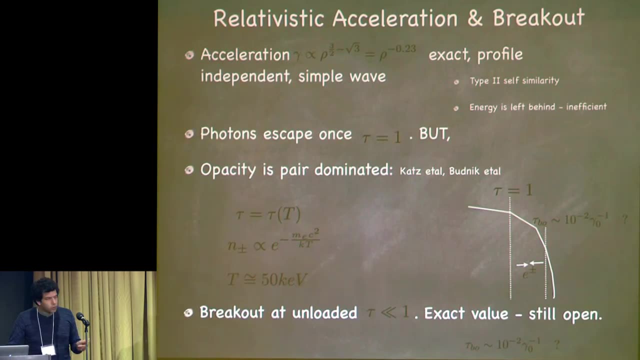 you have a breakout with much higher energies than you would naively assume in equi-partition. So we can talk in more details about how this shock breakout occurs in different environments and how you can calculate everything, but it comes out in the relativistic case. 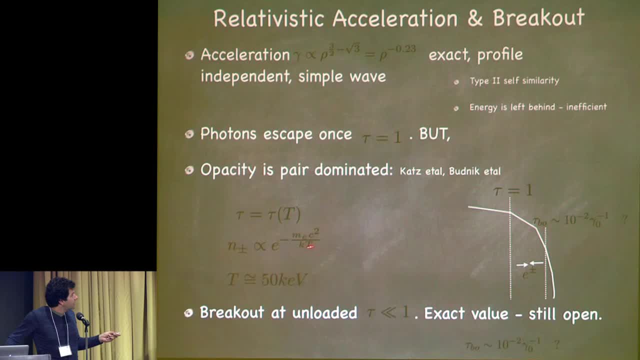 from optical depth of order unity. There is a high loading of pairs when the shock is very fast, but then these pairs annihilate and the radiation leaks out. The temperature in the local frame is said to be something like 50 kV. because this is. 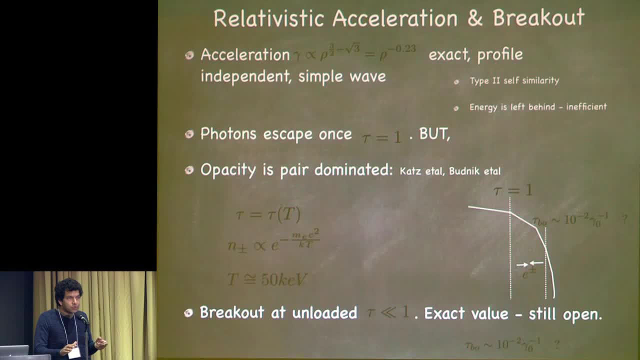 the temperature where most of the pairs annihilate. So regardless of the conditions exactly of the shock, the local temperature is 50 kV. The observed temperature will be 50 kV times gamma. So if you take that simple theory, you have basically two. 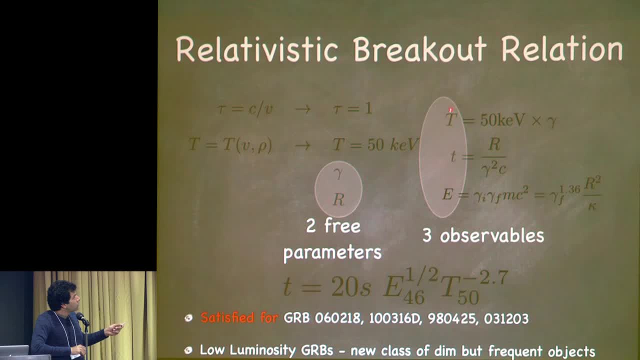 parameters: the Lorentz factor of the shock and the radius of the shock. and you have three observables: The temperature of the photons that you see, which I already told you is 50 kV times. gamma. The duration of the event: the same. 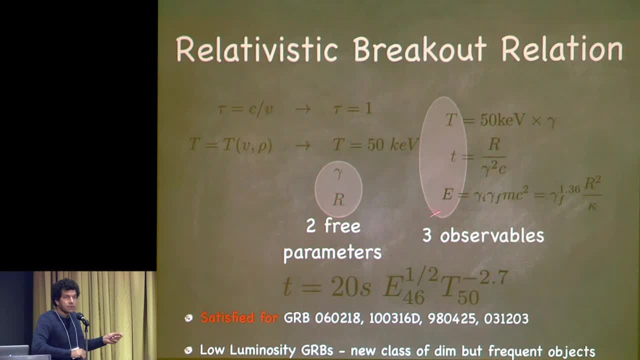 r over gamma squared and the energy of the photons that leaked. It's not exactly the initial energy, because it was degraded by some adiabatic expansion and you lost some, but there is some expression. So you have three observables. 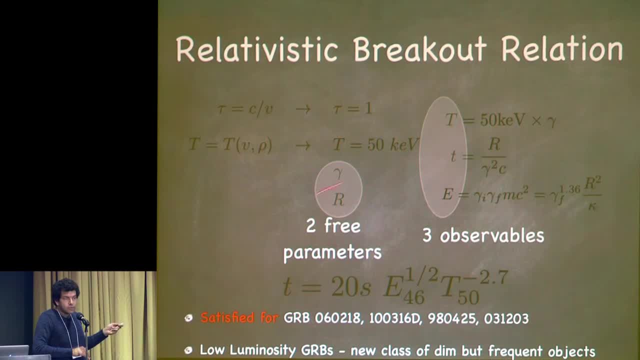 and only two variables in this theory. So the theory is over constraint and you can check if those three observables satisfy this relation. Okay, So if the duration of the burst is proportional to the energy, to the one-half power and to the duration, to the minus three power, 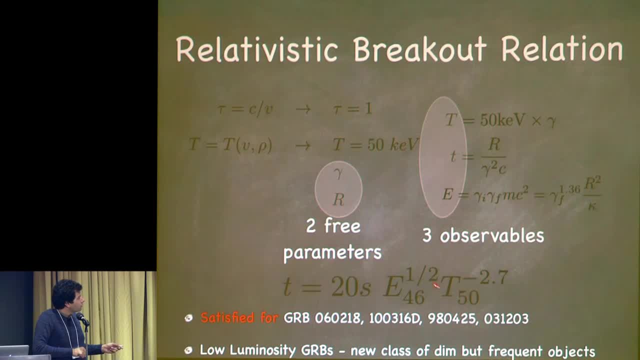 And since the temperature, the observed temperature, to the minus three power. So if we go to the list of bursts that I showed you before, it seems to be roughly satisfied with a Lorentz factor of between one and three for these low luminosity GRBs. 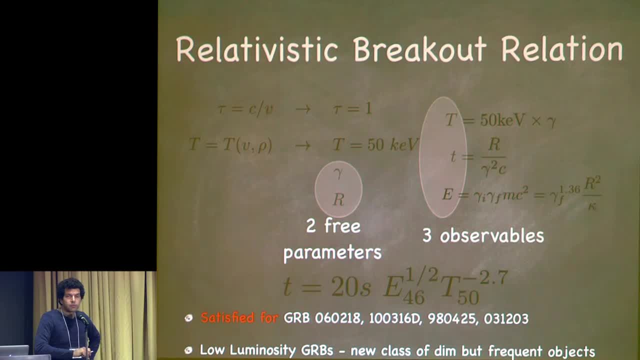 So it's interesting to know if, in the distribution of bursts that we have- and we all think of them as long GRBs, how many more classes like these are there? This seems to be a well-defined class In the real space event. 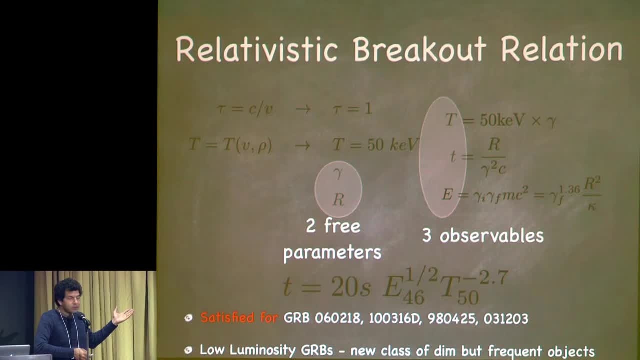 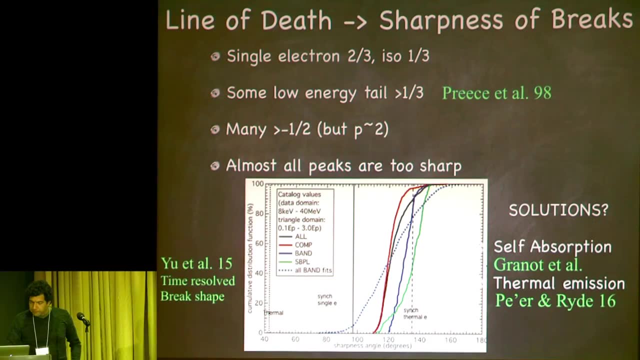 in density of events per unit volume, they seem to be the majority of the events, even more frequent than GRBs, but in the observed ones they are pretty rare. Let me skip that and I'll say that only in the summary. 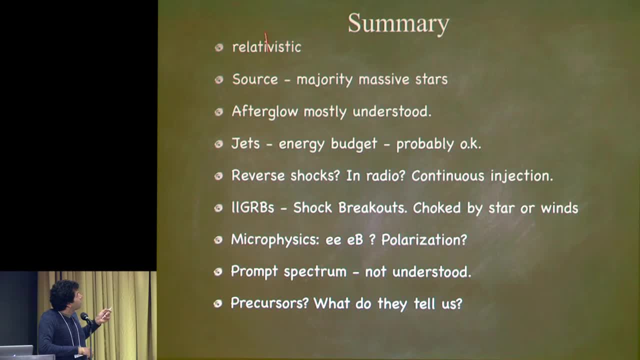 So this is a list of the things I more or less talked about, and I ordered them here in the order of what are we sure of in the long GRB business and what are we less sure of, we know less about? We don't understand the spectrum. 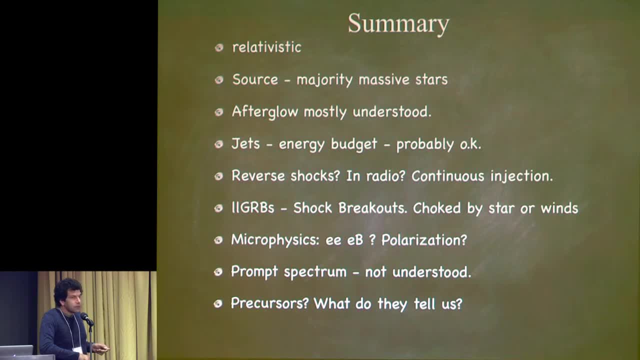 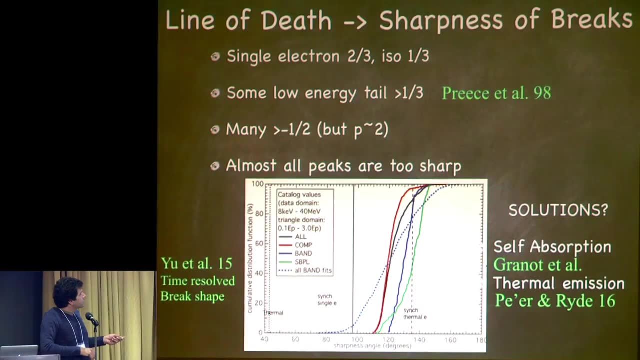 the fact that the spectrum is not thermal. This used to be called the line of death. Maybe I'll put a slide on this. This is a compilation of the sharpness of spectral peaks in GRBs And, instead of measuring the low frequency tail, 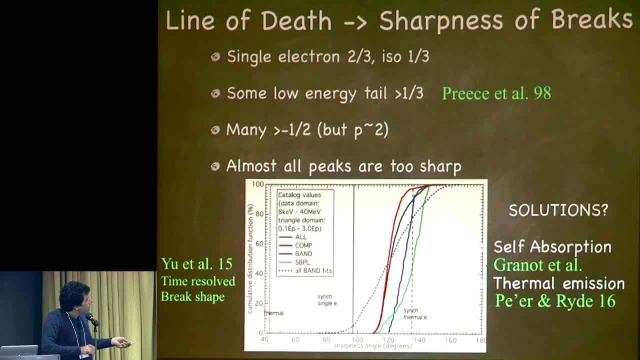 which is so far from the peak that it's hard to analyze. what was measured here is the width of the peak, which is the angle by the peak, And you can see that if you compare that to synchrotron emission, even from a very well concentrated 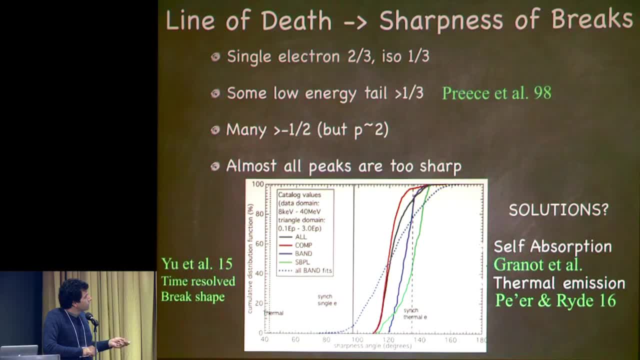 set of electrons not even distributed as a parallel. most of the bursts have spectral features which are wider than that. So I think this problem with the synchrotron radiation for the prompt gamma ray burst itself is real and it's more severe. 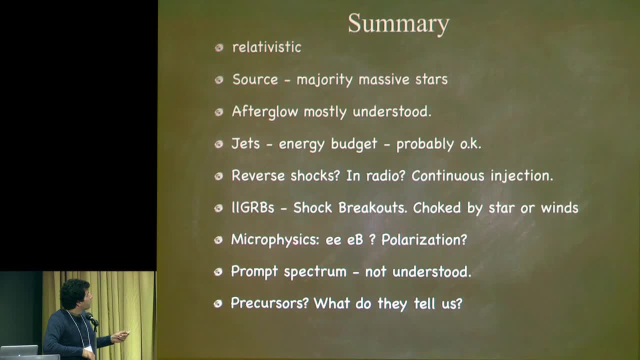 than we thought of before. Low luminosity: I think we more or less understand Reverse shocks. we see them every now and then, maybe not as frequently as I would have expected. Afterglow is well understood, Jets somewhat well. 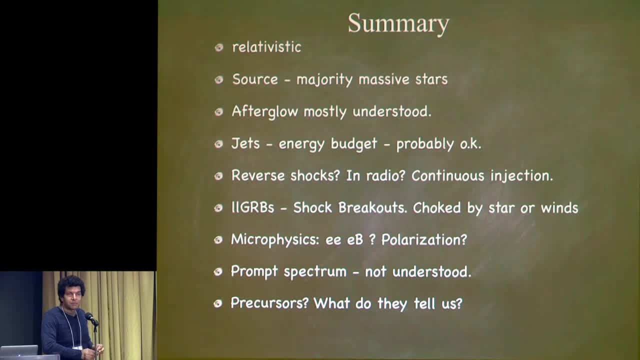 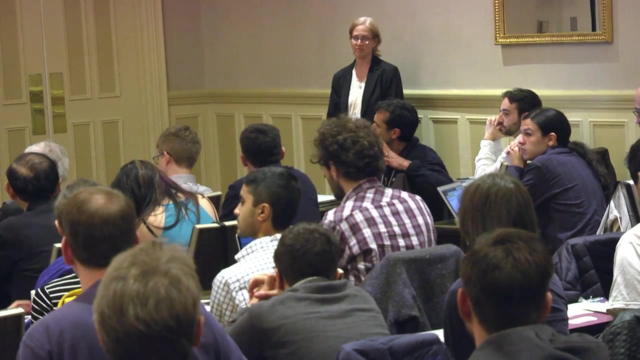 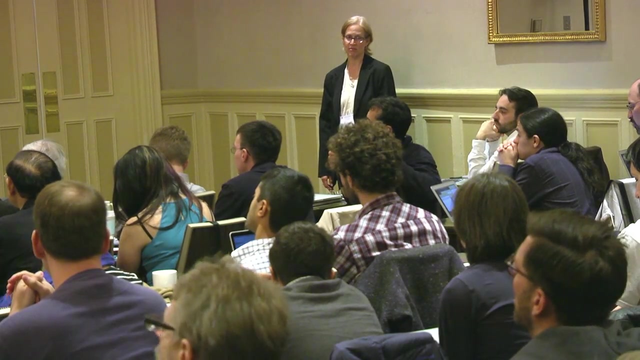 not as well, And I'll end up here. So some long GRBs turn out to be rather smooth or somewhere in between. The standard model of internal shocks kind of gives you some potential for creating this variety, but do you think that it's natural? 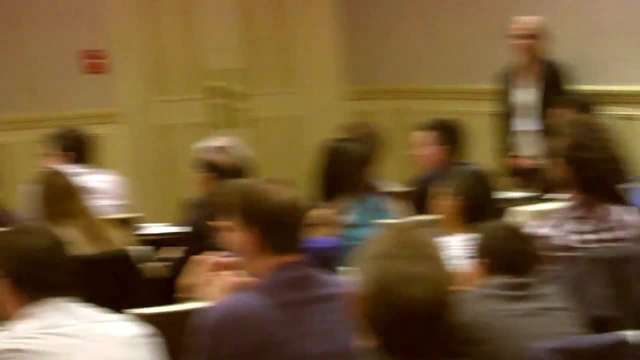 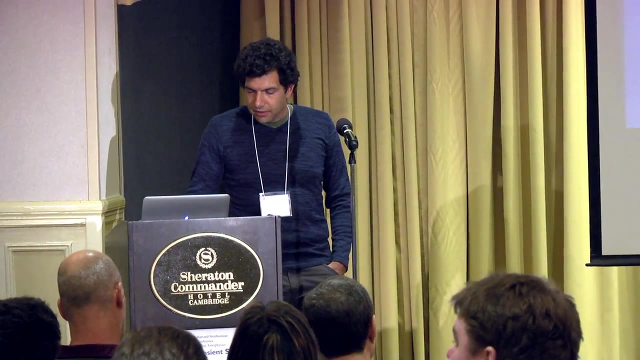 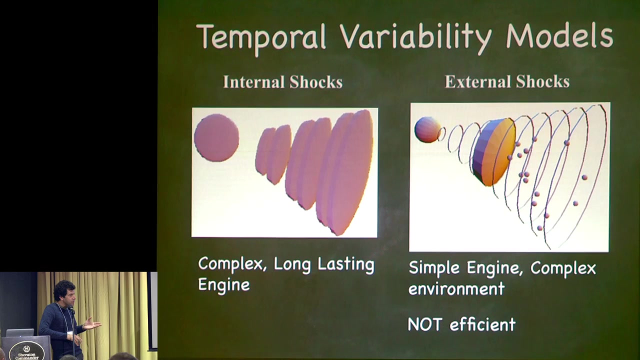 to get such a wide variety in the standard model? You know I don't really understand this complexity. So the fact that you're saying that there is an internal shock model doesn't mean that the burst should be very complex, because it doesn't tell you how many. 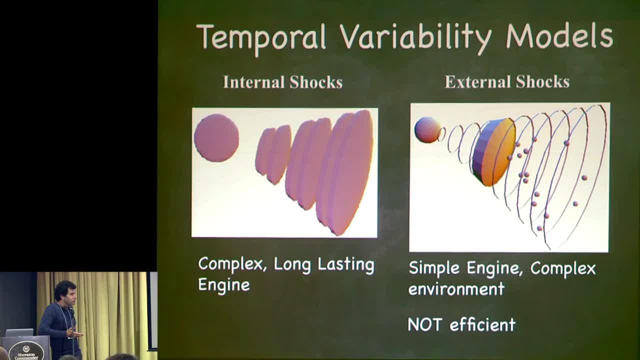 to create all this for you. So I wouldn't know. If you asked me before I would have seen the data. would I expect 100 peaks? I wouldn't. Would I expect just a single one, Maybe. So I would say there is a chance. 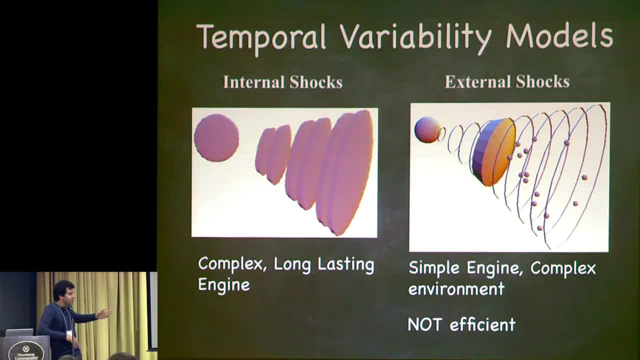 for a variety, but I don't know Now, for example, for the low luminosity GRBs like 98BW or things like that. they are smooth, But we think they are formed in a different way. Some are definitely formed in a different way. 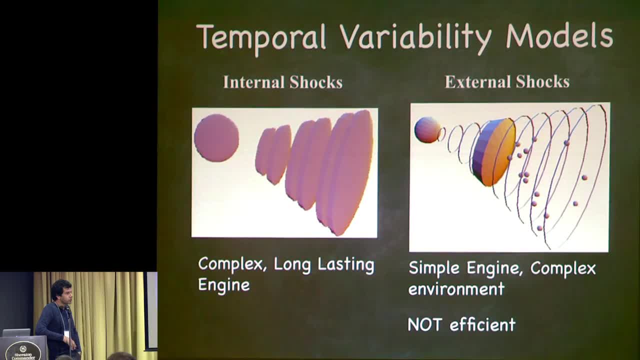 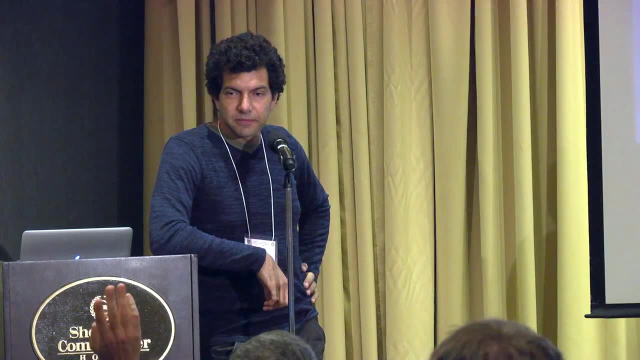 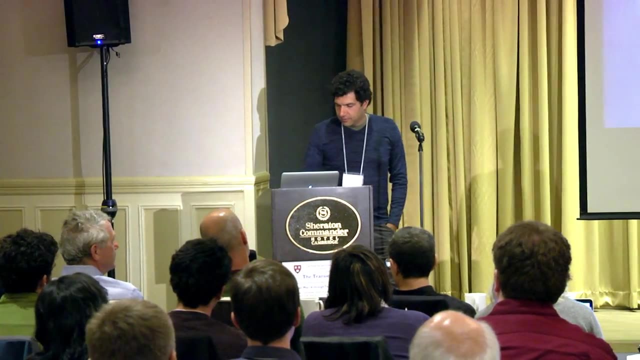 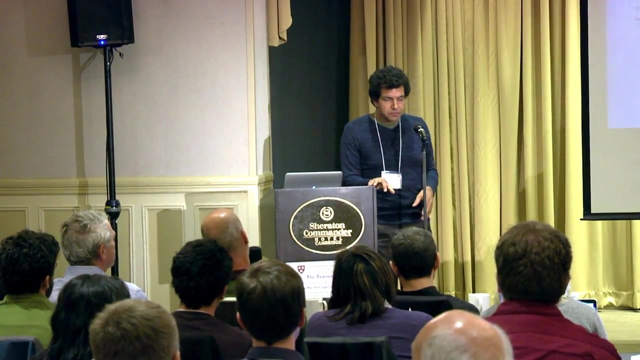 And some could be just internal shocks with fewer shells, therefore smoother. The internal shock in that sense is very unpredictable. You mentioned that the precursors- you would expect them to be thermal from a fireball. Could you explain that? What fireball and why is it emitting gamma rays? 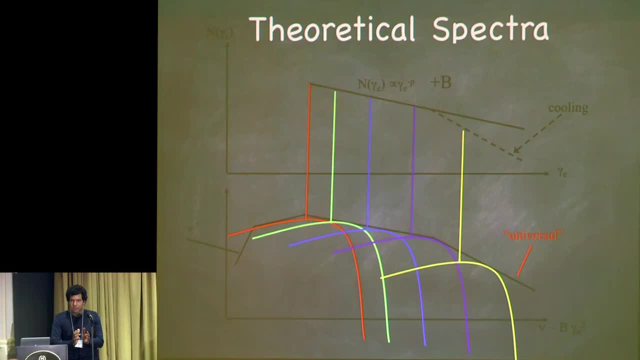 If you take a collection and some pairs and some baryons, you put them in a localized small region, you let the whole thing expand. eventually the fireball will become optically thin As it expands. it will eventually become optically thin. 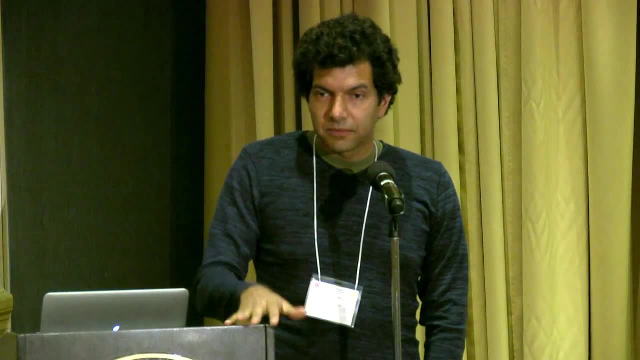 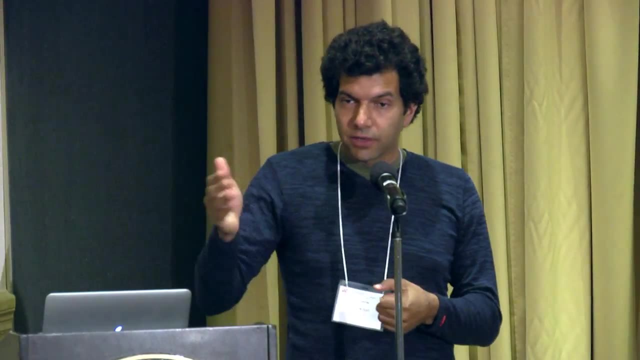 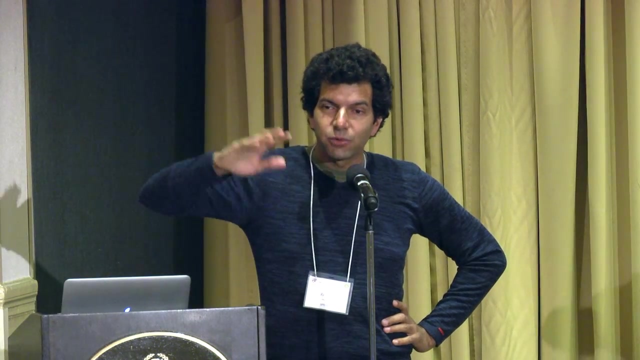 When that happens, the photons that are there, they leak out. Why does this happen? a few minutes before the explosion, So presumably if the internal shocks are doing the, or even the afterglow, the emission, the main emission that you see. 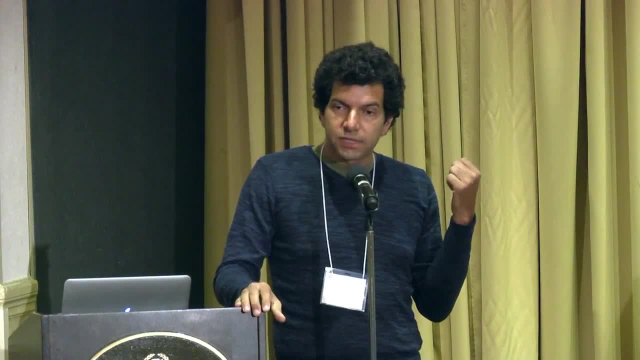 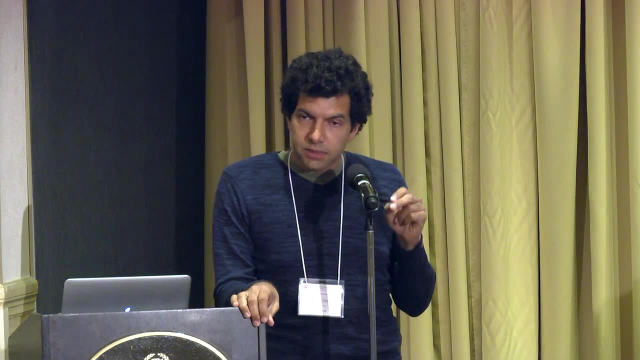 that happens when the things interact either with itself or with the surrounding, and the photons that are coming from the fireball they leak before that And they have to do that before because, if you want the gamma-rebursed spectra itself to be non-thermal, 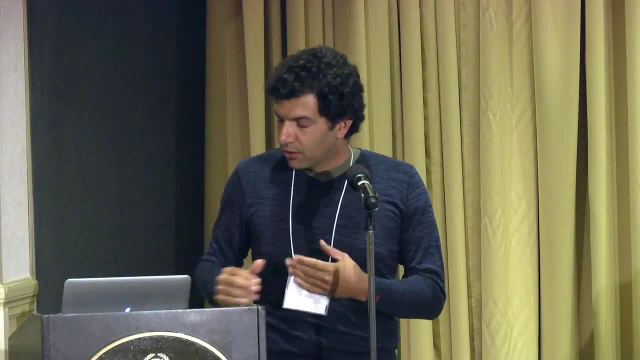 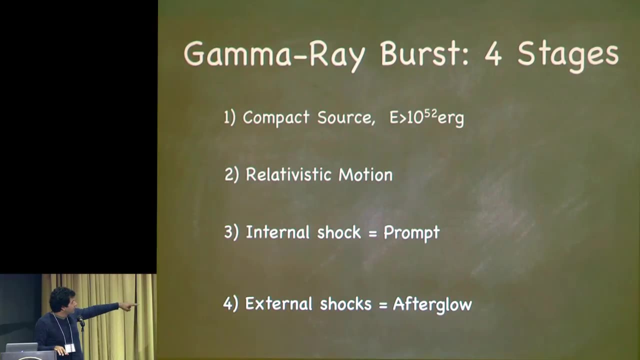 it has to happen when the fireball is optically thin. That was the whole idea in going through this multistage model: here To start with a compact source, but there it's optically thick and you do the internal and external shocks. 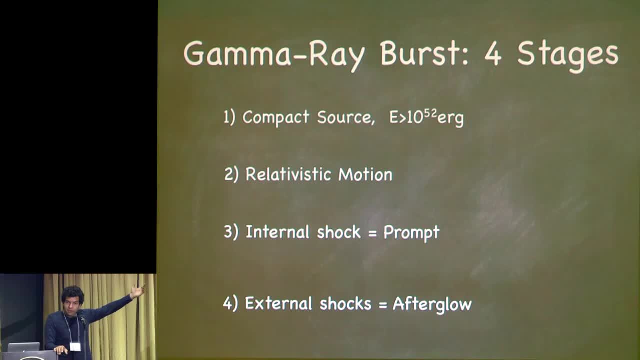 before the spectrum. So somewhere between those there's the position between thick and thin, and it happens before stage three and four. So that's why you expect the precursor to be before Now. some people were claiming that. well, okay, forget this. 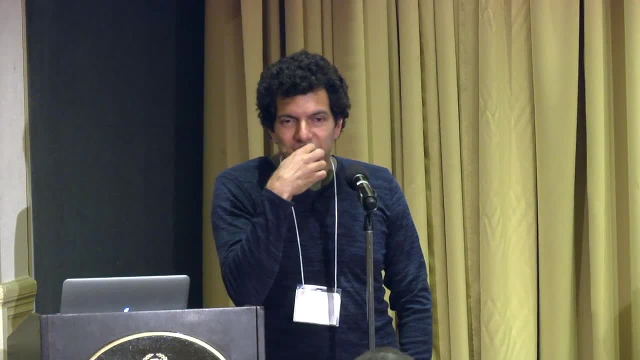 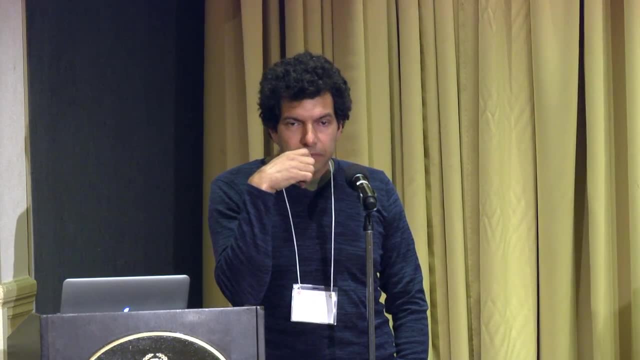 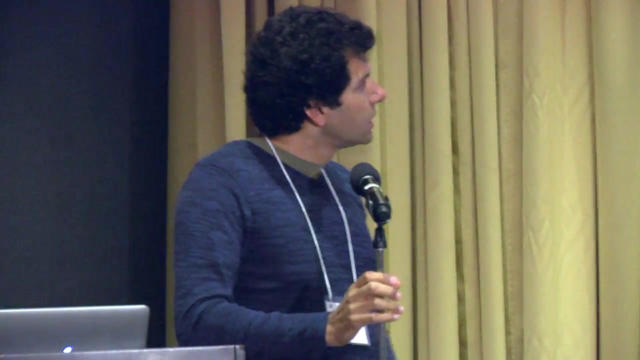 Yes, next second. But at the same time you made the point that the spectrum does not seem to be fit by a parallel population of electrons for the gamma-rebursed itself. So could we just witness the transition region Right, The transition between the two regimes? 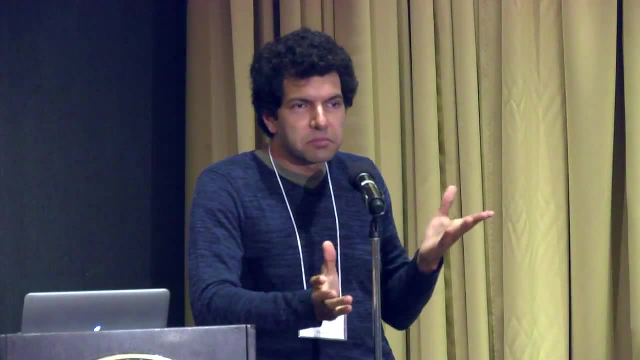 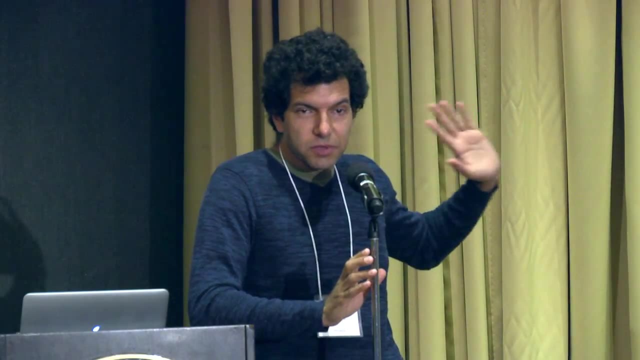 Yes, this is called photospheric emission models and, yeah, I think it may have some merits. I don't really know. Yeah, I was making the point that just synchrotron is not going to work. You have to add either self-absorption.